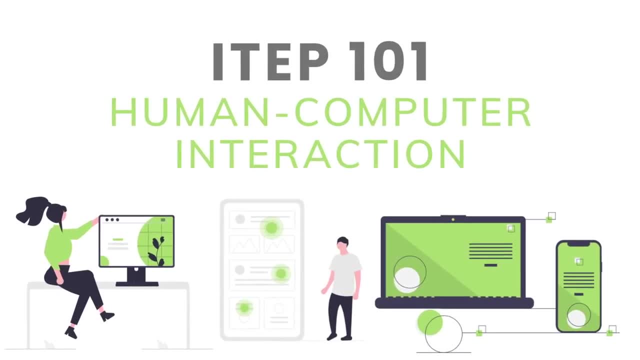 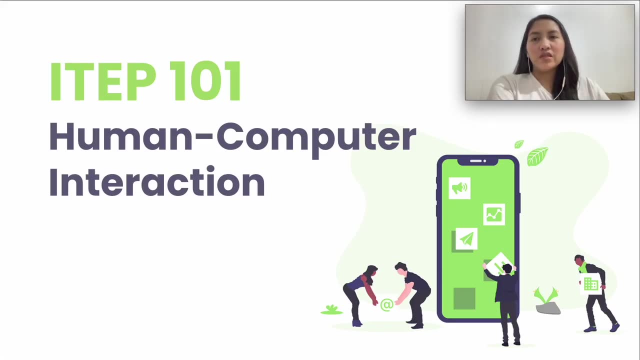 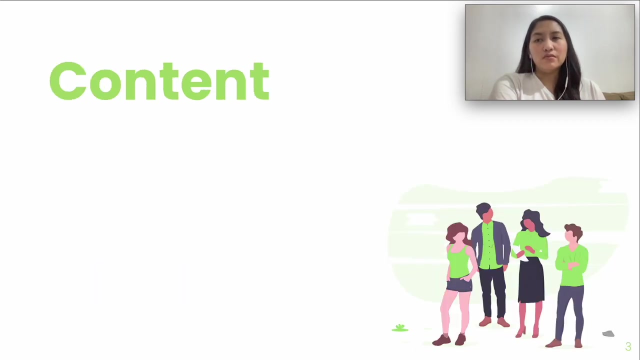 Good day everyone. This is video lesson in ITEP 101, or Human to Computer Interaction. This video lesson will cover the last module, Module 4, which is the lesson entitled Evaluation Techniques. The topics here include Definition and Importance of Evaluation, The Goals of Evaluation, Different Evaluation Methods, Under-Evaluation through Expert Analysis and Evaluation through User Participation. 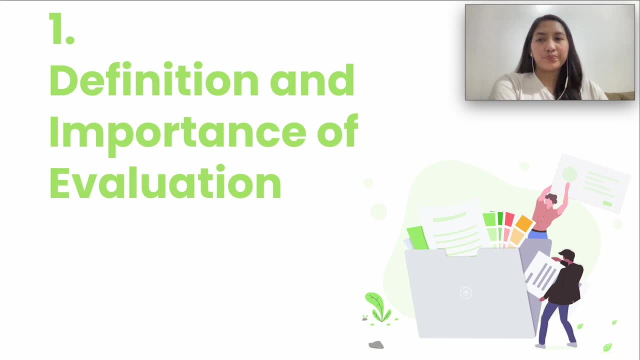 And, lastly, How to Choose an Evaluation Method. What is Evaluation in HCI? Basically, it is the process of judging the usability of a system, interface design and structure based on a set of standards. Evaluation should not be thought of as a single phase in the design process. 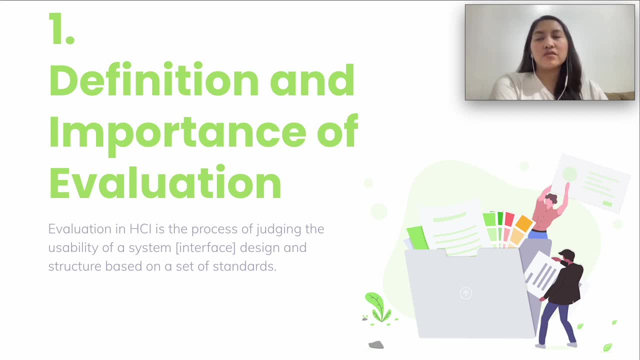 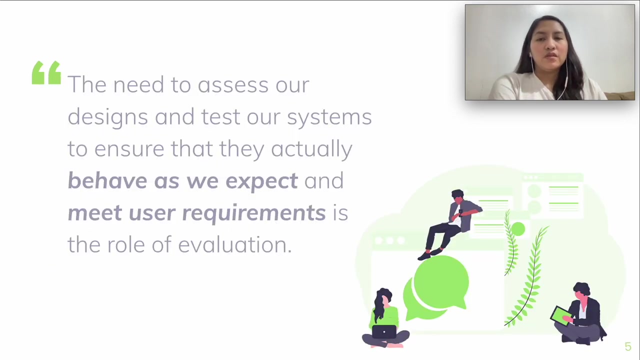 Rather, it should occur all throughout the design lifecycle, with the results of the evaluation feeding back or going back into modifications to the design of the system that is being evaluated. The primary role of Evaluation comes from the need to assess the design and test the system to ensure that they actually behave as expected and if the design have met the user requirements. 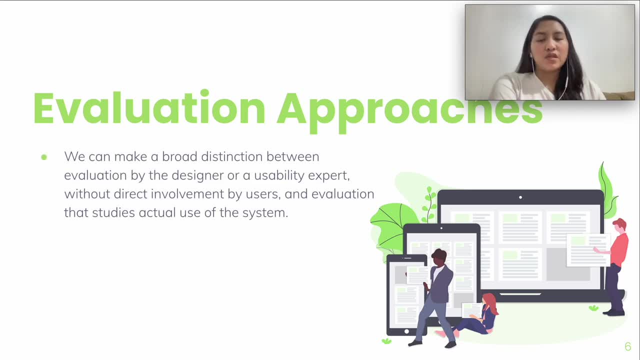 Basically there are two evaluation approaches. There is a broad distinction between Evaluation and Evaluation. Basically, there are two evaluation approaches. There are two evaluation approaches: Evaluation by the designer or usability expert and Evaluation that studies actual use of the system with direct involvement by the users. 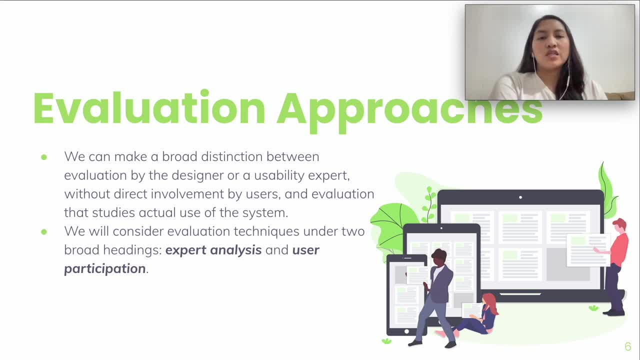 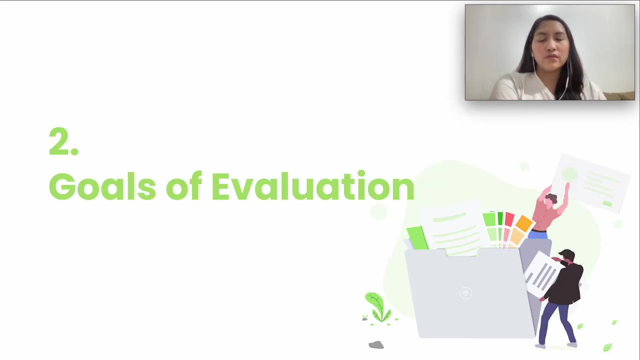 There are several Evaluation techniques that fall under two broad headings: Evaluation through Expert Analysis, Evaluation by User Participation. Evaluation by User Participation. Evaluation by User Participation. There are three goals of evaluation. What are those? So the first one is to assess the extent and accessibility of the system's functionality. 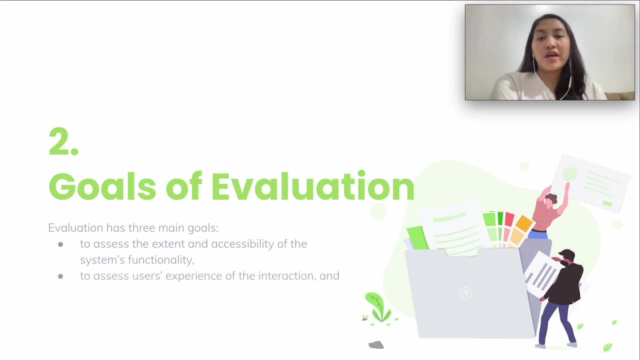 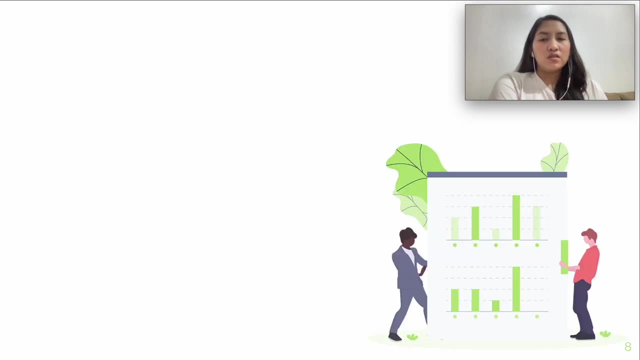 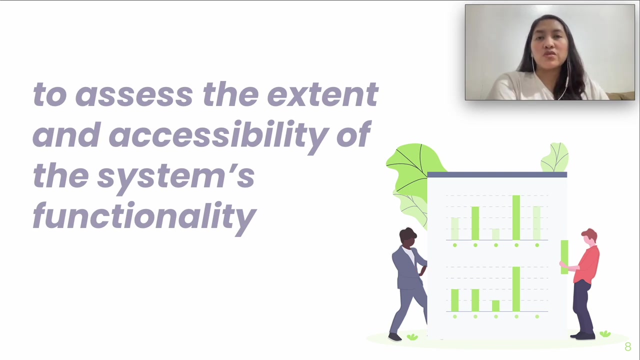 Second is to assess the user's experience of the interaction And, lastly, to identify any specific problems with the system. So let's dive deeper into each goal To assess the system's functionality. So the system has functions that addresses the need and the requirements of the users. 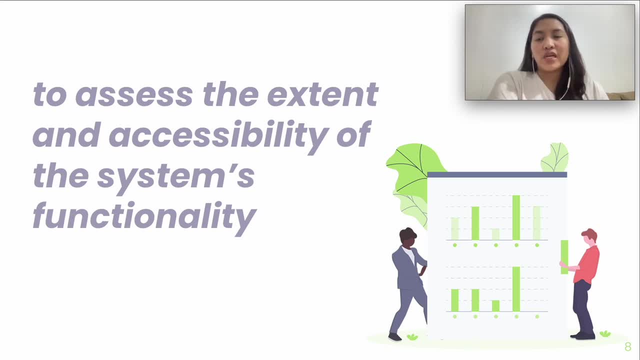 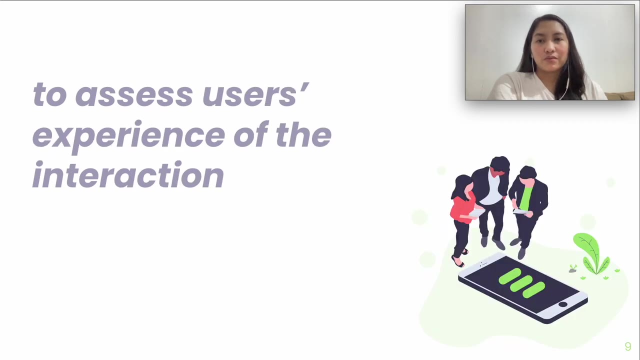 So it is important that the design of the system must be in accordance with the requirements of the users. In other words, the design of the system should enable the target users to perform their intended tasks more easily. Now let's discuss about the second goal: to assess the user's experience. 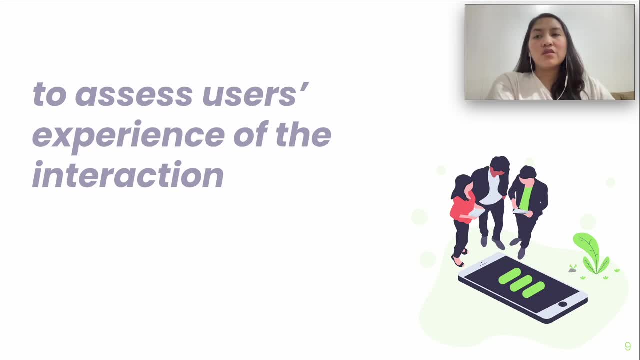 So here we are considering aspects such as how easy the system is to learn, the usability and the user's satisfaction with the design or with the system. Sometimes it may include the level of enjoyment and the emotional response of the user in terms of the system or your design. 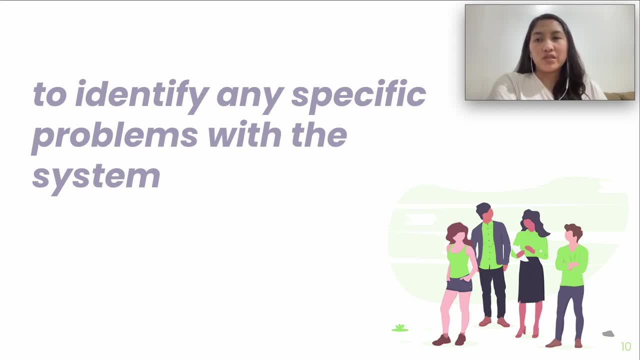 And then, third, to identify any specific problems with the system. So when the intended function of the user or the use of the user produces unexpected results and confusion, there might be some problems that need to be addressed on the design of the system, And this is also addressed by evaluation. 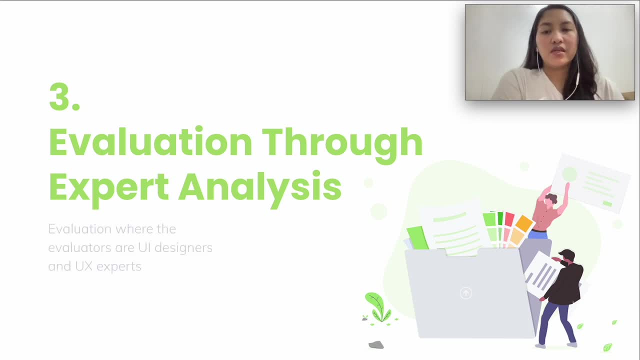 So now let's discuss about evaluation through expert analysis. So this type of evaluation, as the name suggests, is the evaluation where the evaluators are UI designers and user experience experts, or UX experts, So it could be the programmer, the software engineer or the project head. 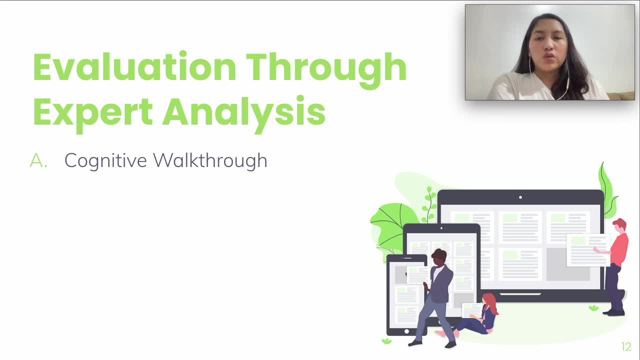 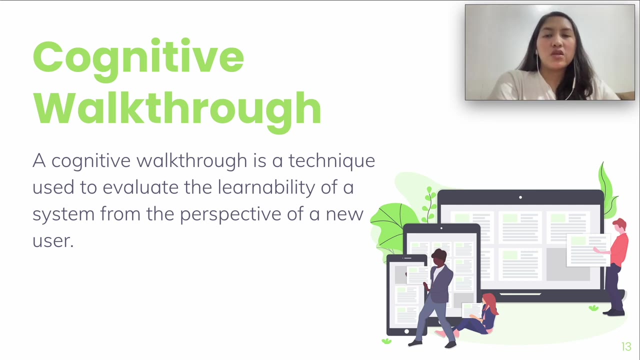 We will discuss two evaluation techniques under this approach. First is the cognitive walkthrough and the second one is the heuristic evaluation. What is cognitive walkthrough? A cognitive walkthrough is a technique used to evaluate the learnability of a system from the perspective of a new user. 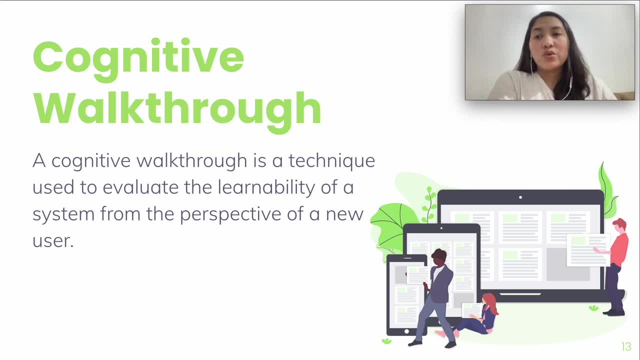 So, unlike user testing, it does not involve the users and thus it can be relatively cheap to implement Here. the expert reviews relies on the expertise of a set of reviewers who, in a highly structured manner, walk through a task or a set of tasks to assess the interface from a new user's point of view. 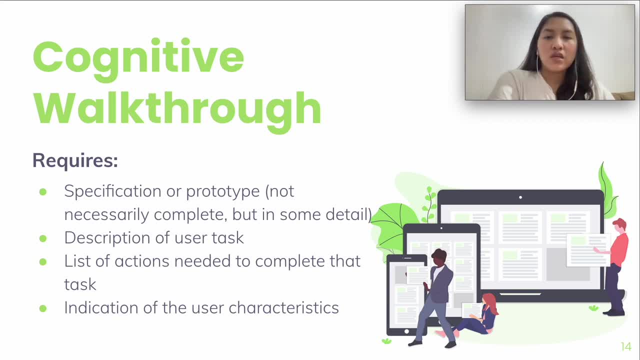 In cognitive walkthrough. we need specification or prototype of the system. It doesn't have to be complete, but it should be fairly detailed. Details such as the location wording for a menu can make a big difference. Second, a description of the task that the user is to perform on the system. 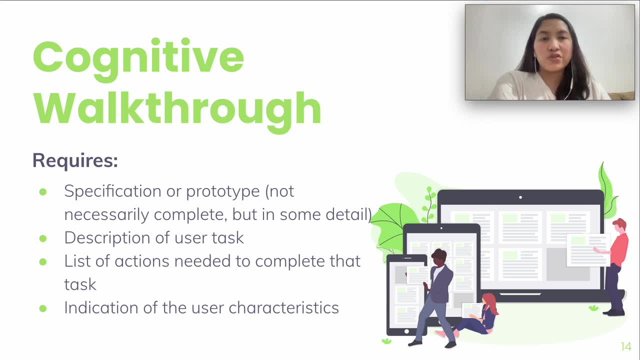 So this should be a representative task that most users will want to do, such as the major functions that the system gives to the user. Third, a complete written list of the actions needed to complete the task with the proposed system. And, lastly, an indication of who the users are and what kind of experience and knowledge the evaluators can assume about them. 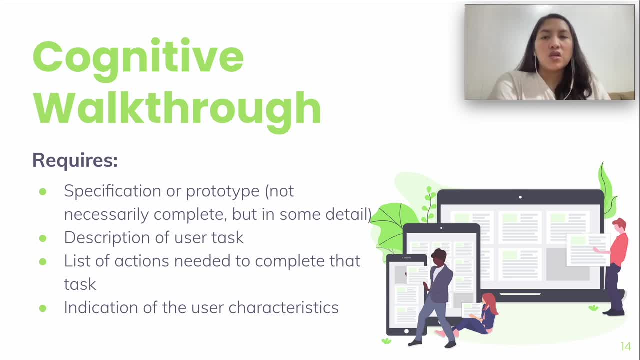 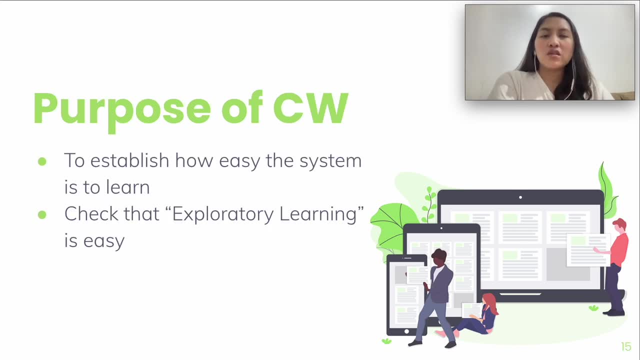 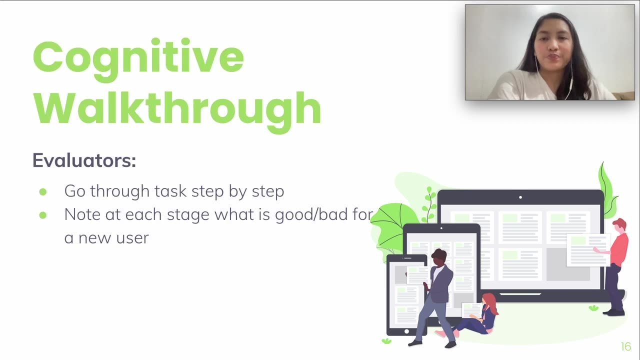 So with the presence of these four requirements, you can now conduct cognitive walkthrough. The primary purpose of cognitive walkthrough is to establish how easy it is to see the system is to learn, or to check the learnability of the system. So here in cognitive walkthrough, the evaluators go through the task step by step. 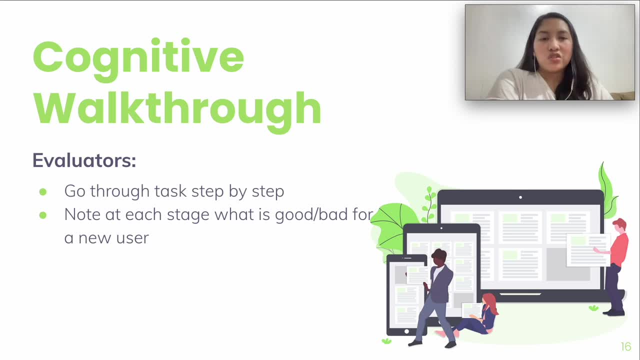 And then he or she will note at each stage what is good or bad for a new user. And he needs to answer four questions. First, will users try to achieve the right result? It must be answered by yes or no. Every task that the evaluator must test must be answered by the evaluator himself with either yes or no. 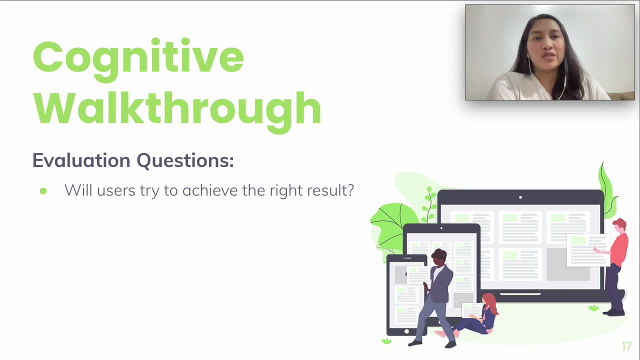 Or he can also note some details about what's wrong or what's right about the interface being evaluated or a task being evaluated. The second question is: will users notice that the correct action is available? So these two must be answered by either yes or no, and can take notes on why yes or why no. 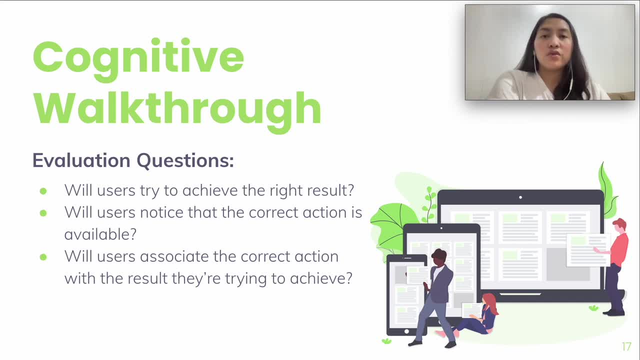 Third evaluation question in cognitive walkthrough that the evaluator must answer is: will users associate the correct action with the result they're trying to achieve? So there must be an indicator that the action was accepted by the system. This is also answerable by yes or no and having notes for details about the answer of the evaluator. 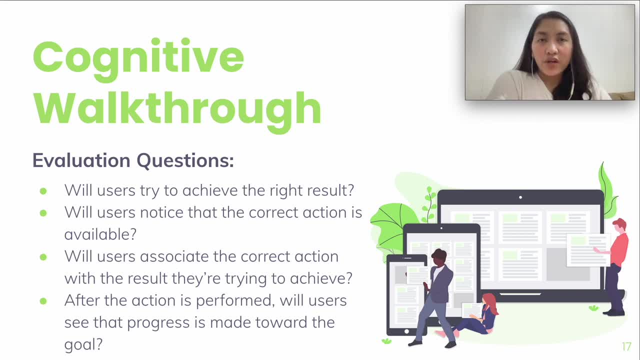 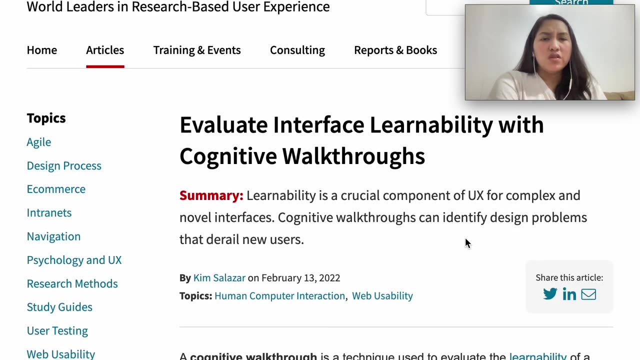 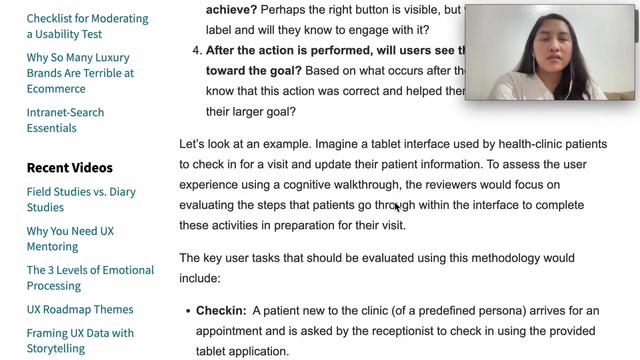 So after the action is performed- this is the fourth question- will users see that progress is made toward the goal? So it is closely related with the third question. Let's proceed to an example of a cognitive walkthrough. So here an interface of learnability is evaluated using cognitive walkthrough in a system related to the medical field. 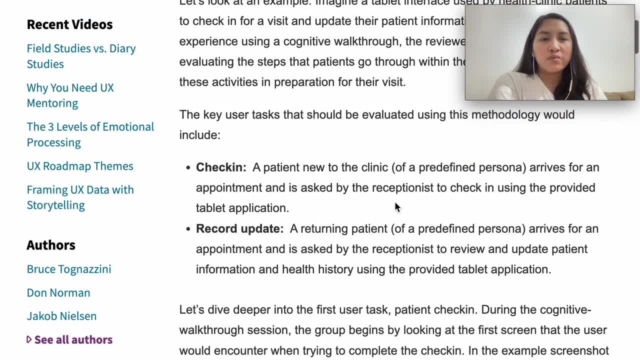 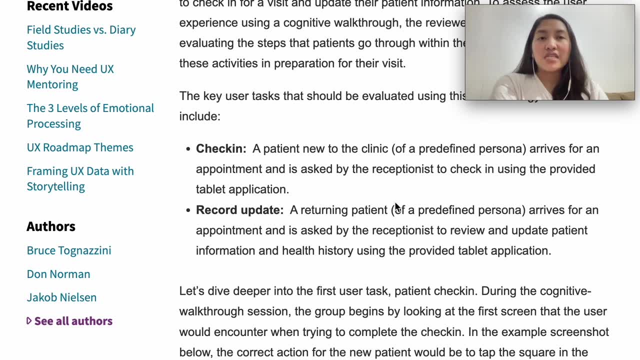 So here there are two tasks that will be evaluated, and then the expert user will play as a new user. He will pretend as if he is a new user, based on the learnability of each task or the different factors in an interface being evaluated. So in this case, two tasks will be evaluated: check-in and record update. 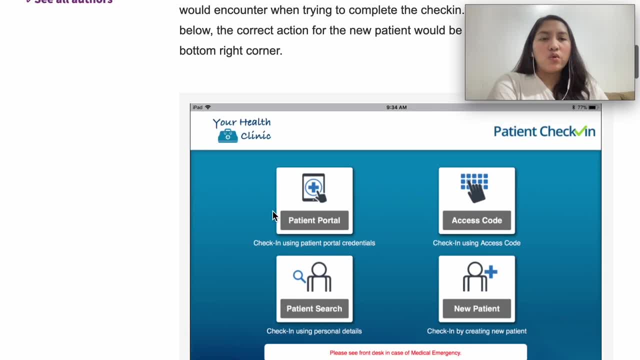 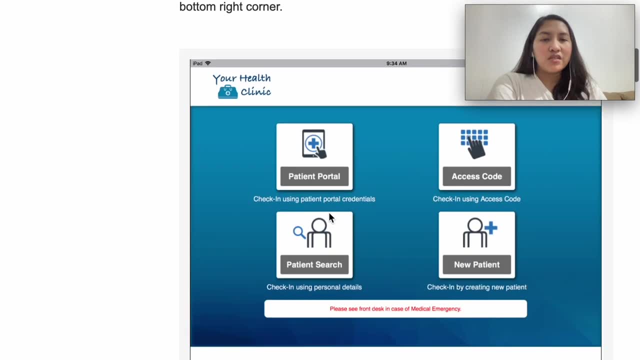 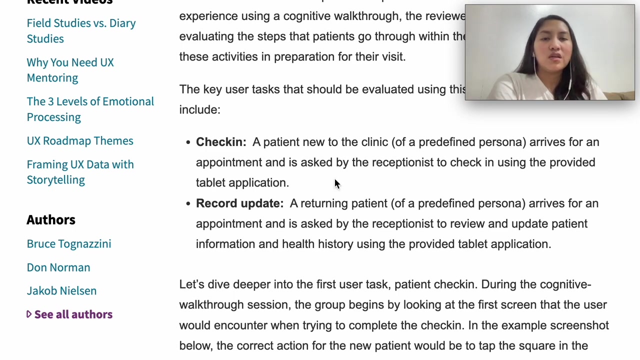 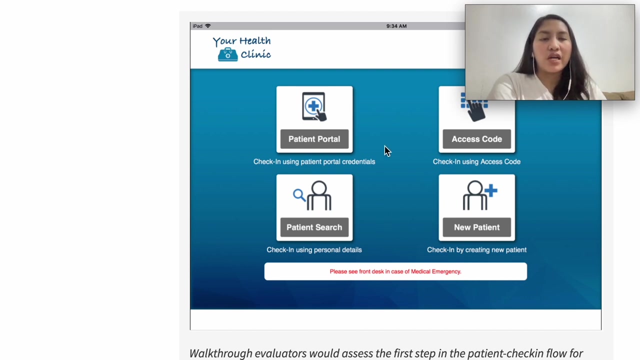 So here there is a system where the interface is an iPad interface and then the receptionist will hand over this interface to the user and then he will let him check-in. If he is a new user or a new patient to the clinic, then every patient needs to check-in to the portal and give his or her information. 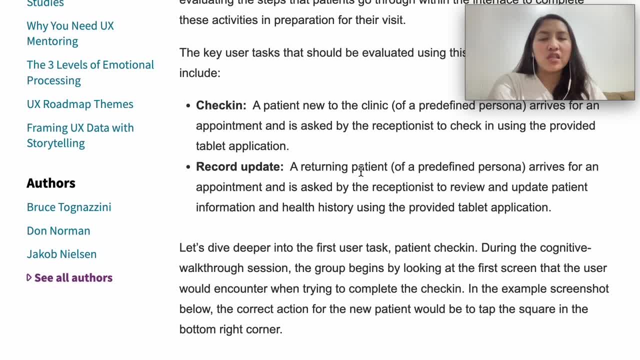 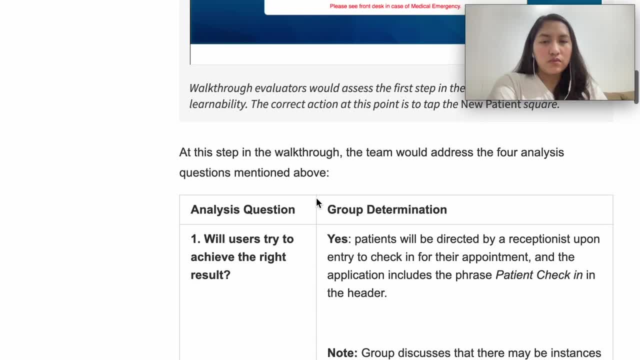 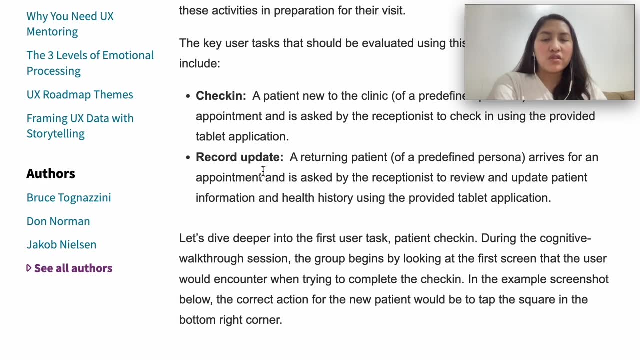 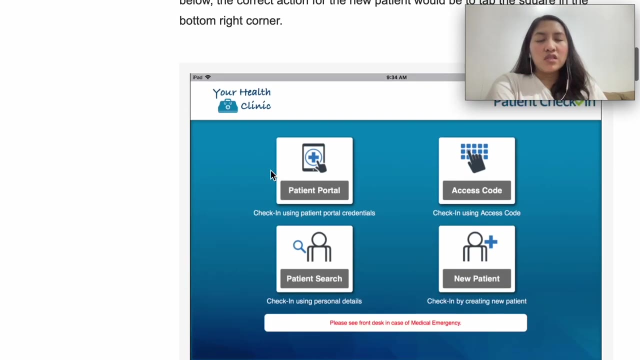 Now, if a patient is a returning patient, then all he has to do is to update the record. So, since we have a task at hand, so we have check-in and record update, the evaluator will serve as a patient in this cognitive walkthrough session. 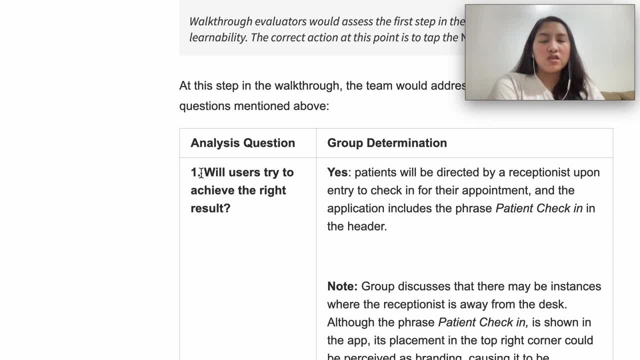 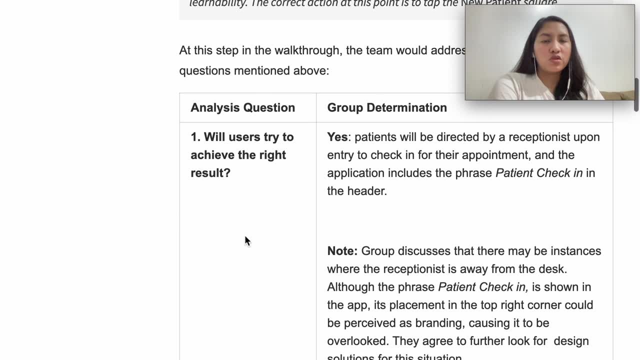 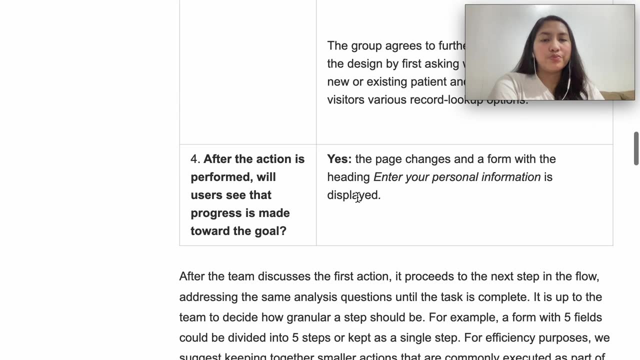 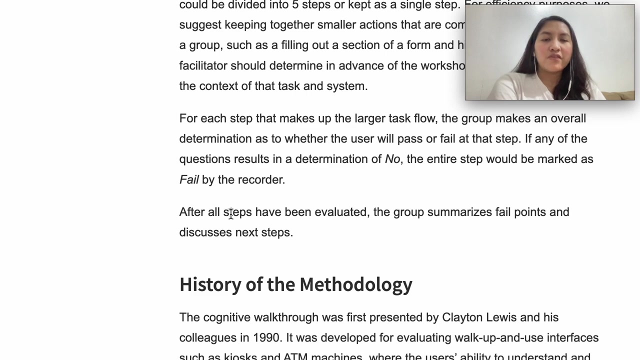 So he needs to answer the questions: the first question, the second, the third and the fourth question with regards to the first task, So with either yes or no, having notes on why yes or why is it no, And then, basically, after all the steps have been evaluated. 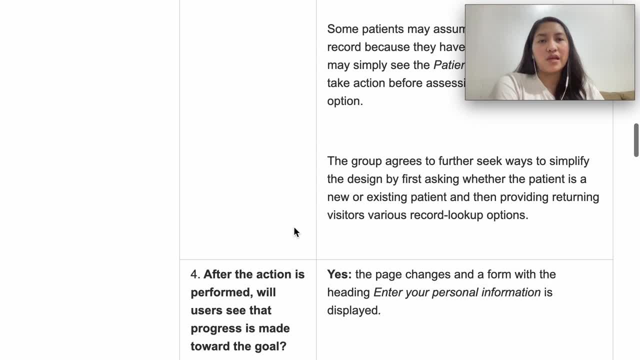 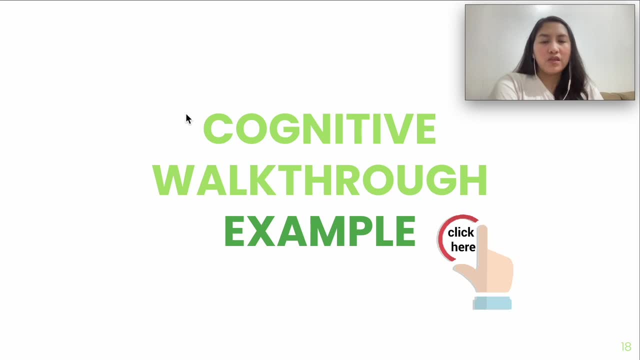 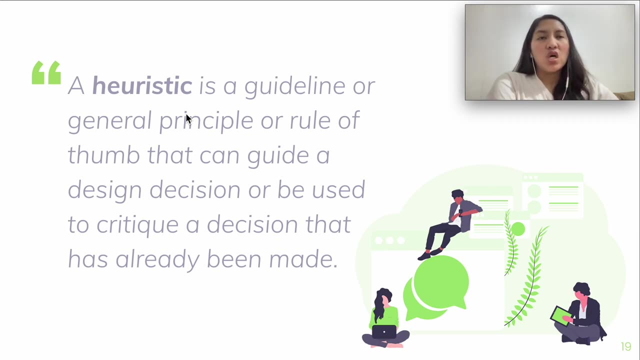 the group summarizes fail points and discusses next step based on their answer to the four questions. Okay, so that's it for our example of cognitive walkthrough. Now let's discuss about the second example of evaluation by expert analysis, which is the heuristic evaluation. 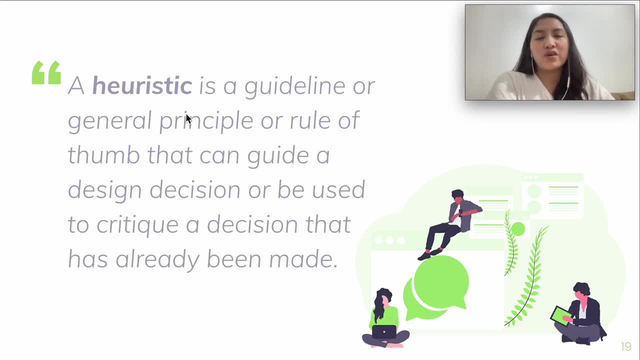 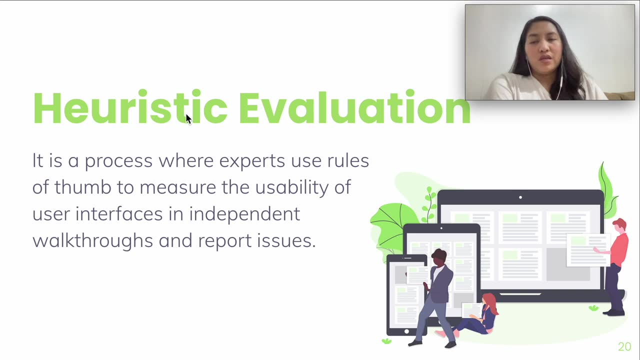 When you say heuristic, it is a guideline or general principle or rule of thumb that can guide a design decision or be used to critic a decision that has already been made. Heuristic evaluation is a process where experts use rules of thumb or heuristics. 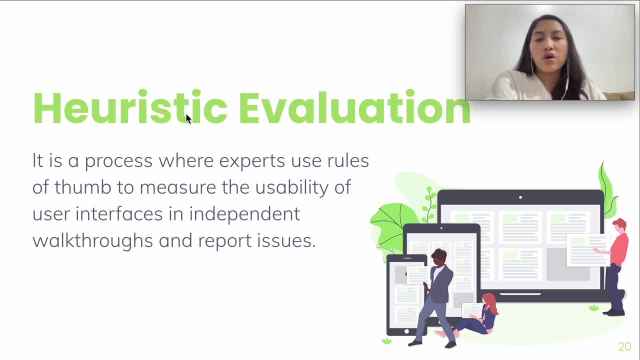 to measure the usability of the user. They use the usability of the UI in independent walkthroughs and report the issues. The evaluators: they use established heuristics such as the Nielsen and Molex heuristics and reveal insights that can help design teams enhance product usability from early in the development. 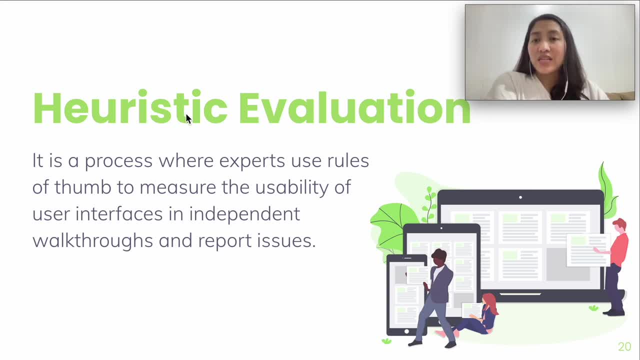 The general idea behind heuristic evaluation is that several evaluators independently critique a system to come up with potential usability problems. It is important that there be several of these evaluators and that evaluations be done independently so that their collective insights will really be useful in the improvement of the user interface being evaluated. 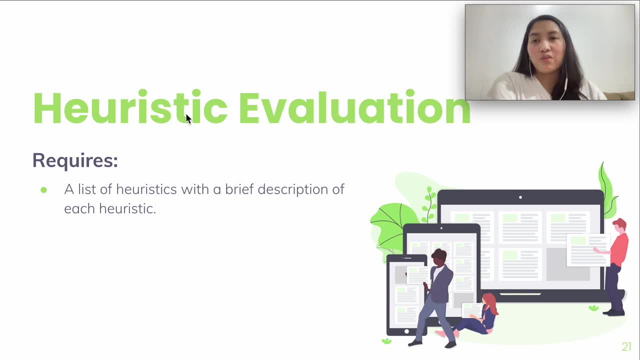 So heuristic evaluation requires a list of heuristics with a brief description of each heuristic, a list of tasks and or components of the product that you want inspected. So, for example, for a major website, you might designate 10 tasks plus 10 pages that you want reviewed. 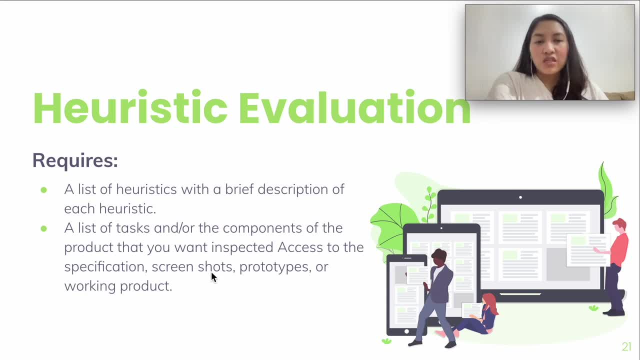 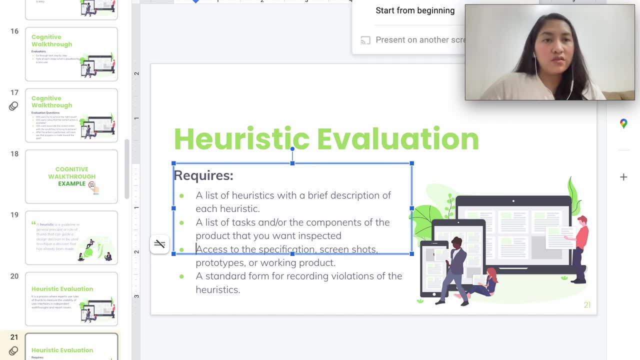 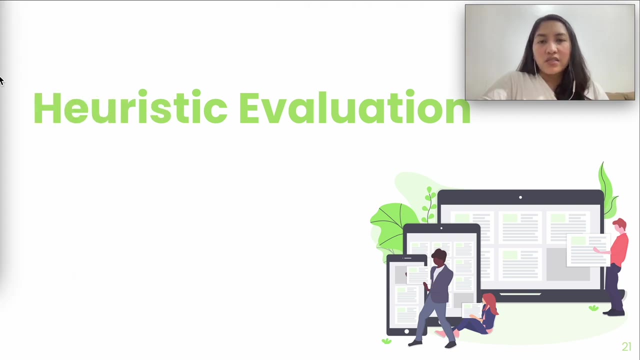 So the next is access to the specification, screenshots, prototypes or working product. So let me just edit this in a while. So here, as you can see, a list of heuristics, a list of tasks, access to the specification, screenshots or prototypes or a working product. 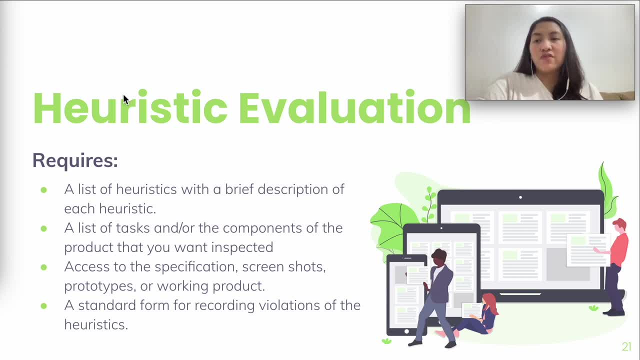 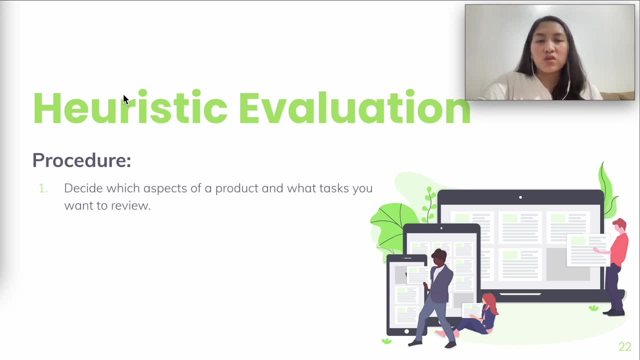 and a standard form for recording violations of the heuristics. So for the procedure, you have to decide which aspect of a product or what task you want reviewed. So you must have a list of tasks you want to evaluate And then you have to decide which heuristics you will use. 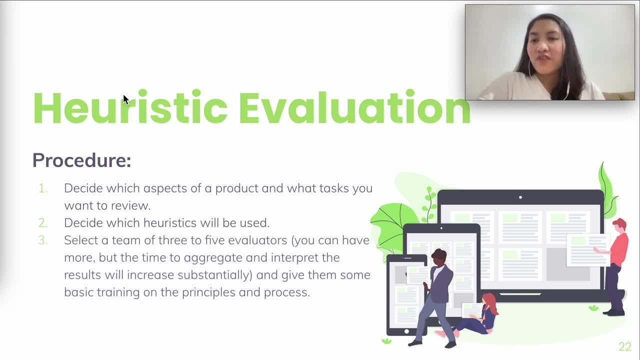 And then, second, you have to select a team of 3 to 5 evaluators and give them some basic training on the principles and the process of the heuristic evaluation. So you should explain to them the heuristics that you chose And then create a list of representative tasks for the application or component you are evaluating. 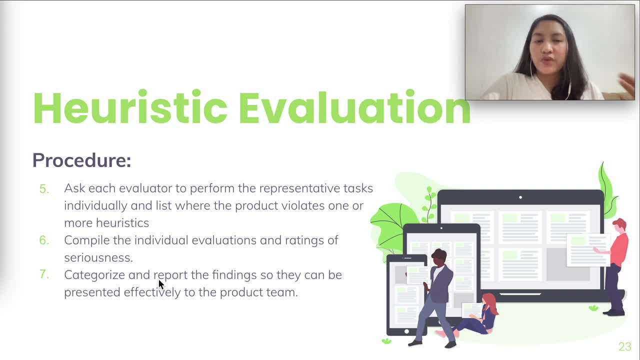 And then you have to ask each evaluator to perform the representative task individually and list where the product violates one or more heuristics. And then you have to compile the individual evaluations and ratings of seriousness, because every evaluator will rate every issue that has been uncovered. 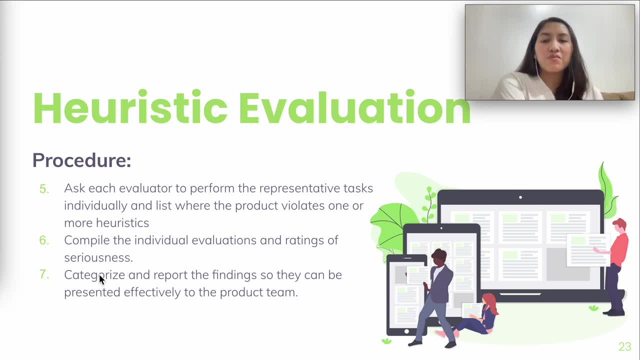 Lastly, you have to categorize and report the findings so they can be presented effectively to the product team. So all of these issues and the ratings of seriousness of these issues will be presented to the designers or the product team and then they will do something about it. 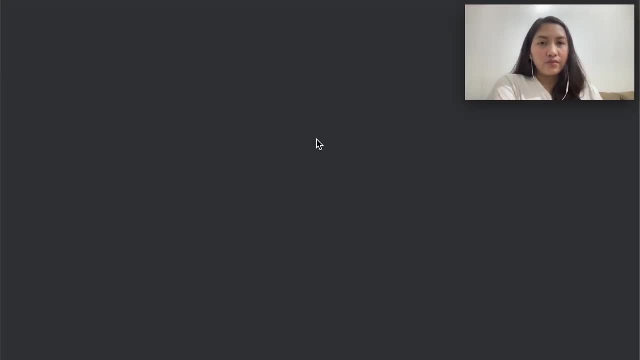 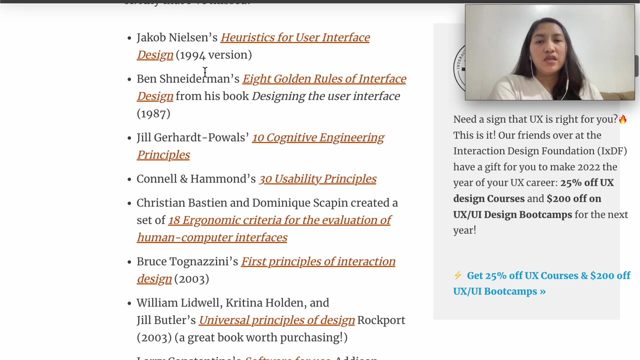 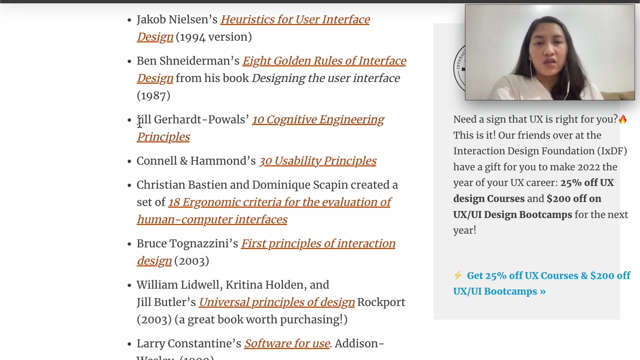 So there are different heuristics available. Okay, so we have here a list: The Jacob Nielsen Heuristics for User Interface Design. The Schneiderman's 8 Golden Rules of Interface Design. 10 Cognitive Engineering Principles by Jill Gerard-Powles. 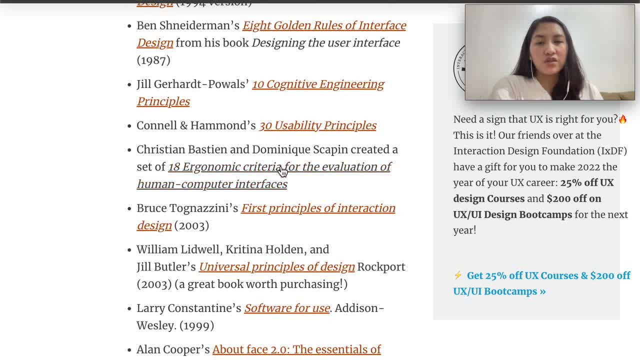 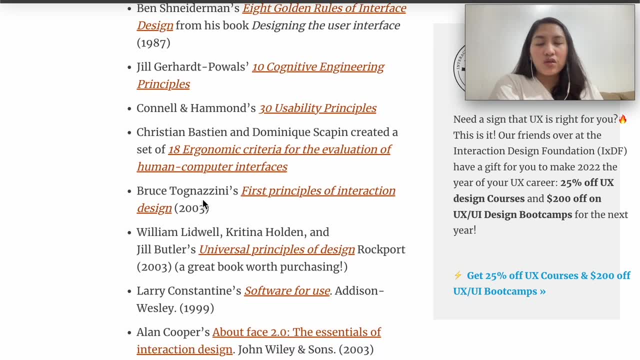 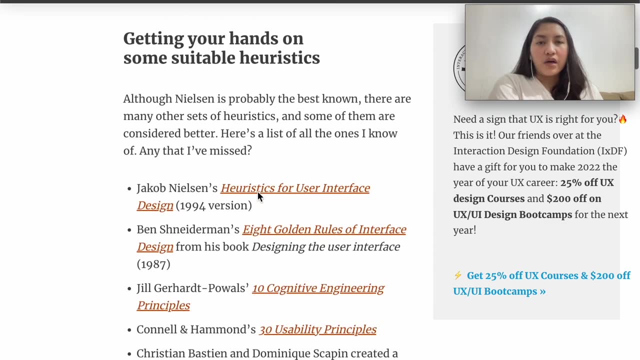 30 Usability Principles, 18 Ergonomic Criteria for the Evaluation of Human-to-Computer Interfaces, The first Principles of Interaction, Design by Prus Tognasinis And among many others. So you can visit this link for to check on the different. 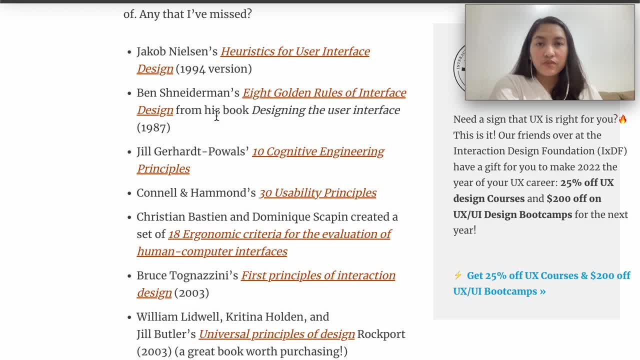 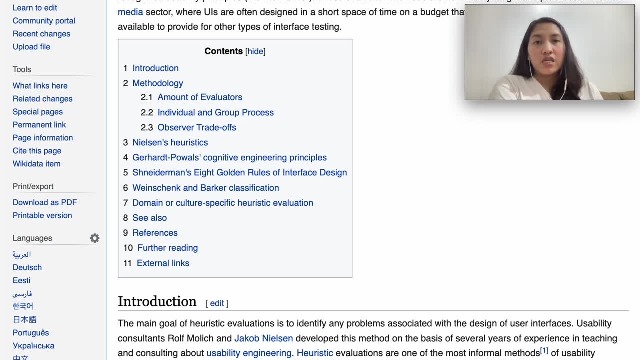 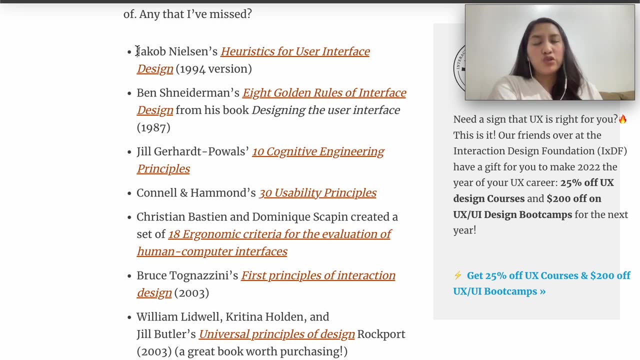 heuristics available. Okay, so here it's. we don't have only one heuristic available, We have many. So we can utilize all of this Well, depending on the need. So you have to really carefully choose which heuristics you are going to use. 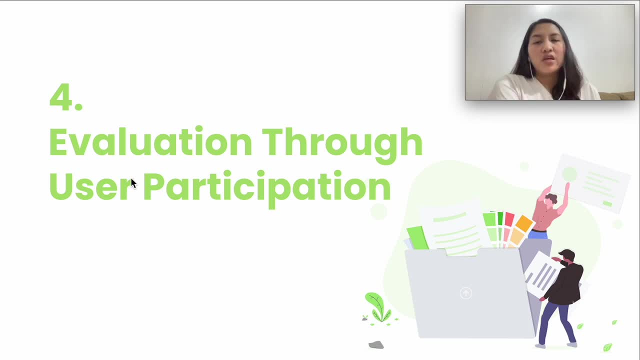 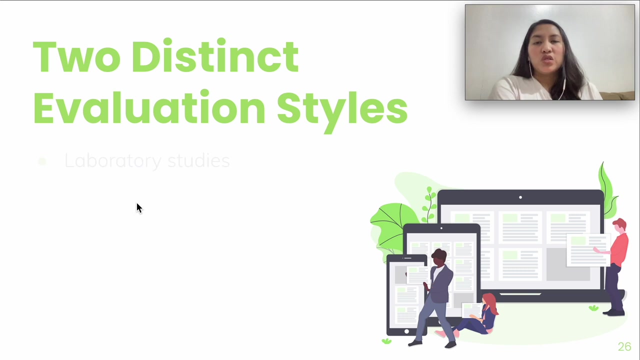 Okay, so let's go back Now. let's proceed to the Evaluation through User Participation. So we have empirical methods, observational techniques and query techniques. So with each approach here there are evaluation techniques that can be used for every approach. Okay, so there are. 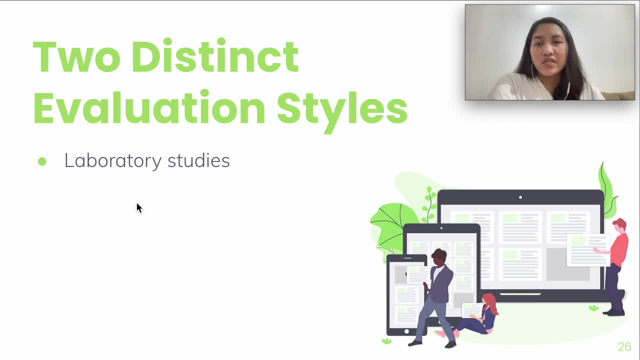 two different evaluation styles: The first is Laboratory studies And the second is the Field studies. Okay, so the laboratory studies studies, these are the evaluation techniques performed under laboratory conditions. And then for the field studies, these are the evaluation techniques conducted in the work environment or 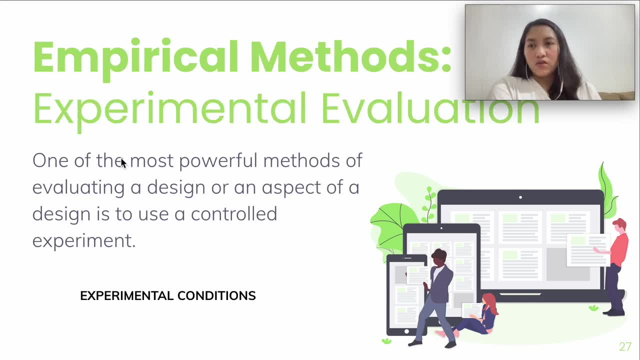 in the field. Okay, so let's discuss about the empirical methods. So we have the experimental evaluation. This is one of the most powerful methods of evaluating a design or an aspect of a design is to use a controlled experiment. So an experiment has same basic form. So we have. 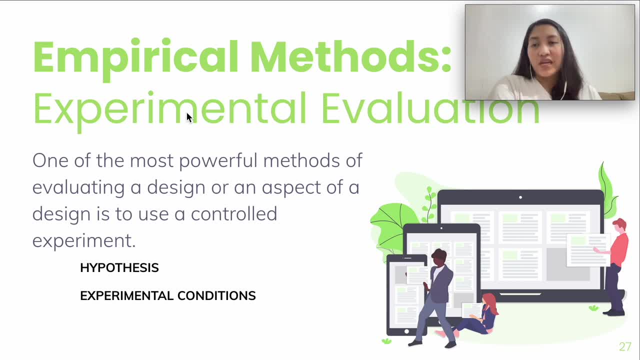 the evaluator chooses a hypothesis to test which can be determined by measuring some attribute of participant behavior. So first we have hypothesis and then you also have a number of experimental conditions which you will apply on the system, And therefore you have controlled behavior, And then you also have a number of experimental conditions which you 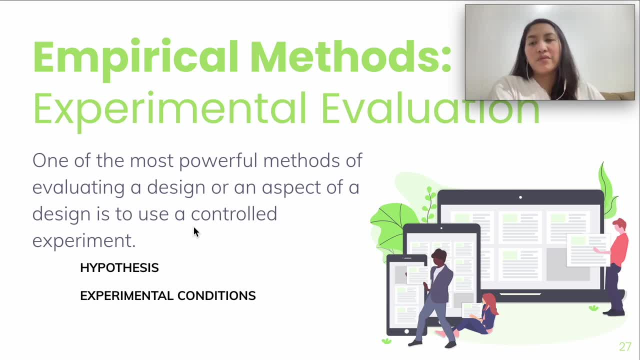 will check on the variables And you will check on the behavior of the system upon applying those conditions or controlled variables. Within this basic form, there are a number of factors that are important to the overall reliability of the experiment. Remember that this is an experiment. 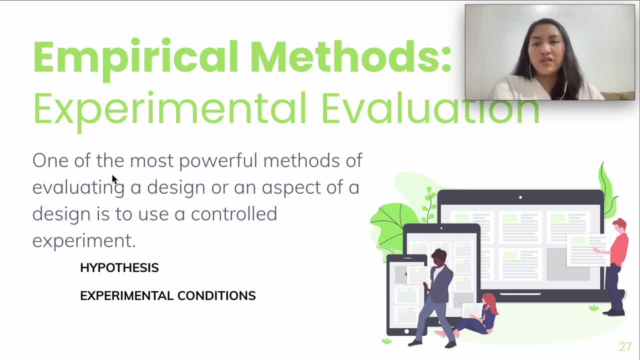 Okay, So this includes the participants chosen, the variables tested and manipulated and the hypothesis being tested. So if you are going to apply this kind of evaluation method, you must know your hypothesis, You must have some experimental conditions that will be applied to. 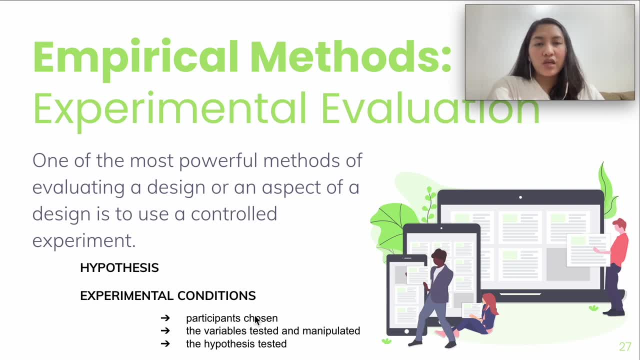 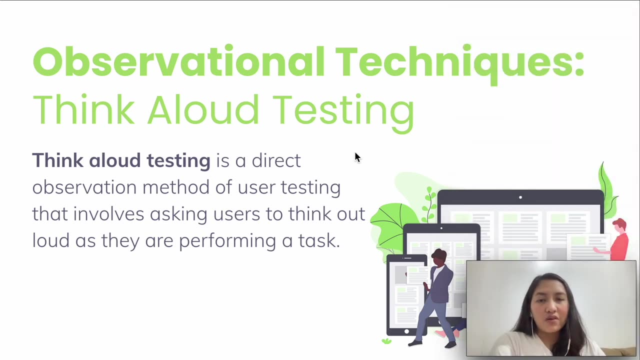 the system or the UI, And it will. the experiment will depend on the participants chosen, the variables tested and manipulated and the hypothesis being tested. Next we have the observational technique. So the first one is the think aloud testing. This technique is a direct 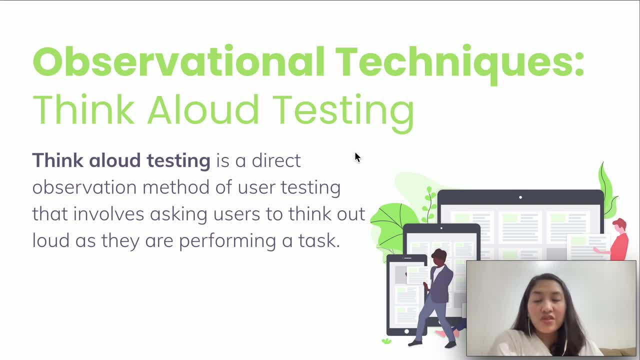 observation method of user testing. that involves asking users to think out loud as they are performing a task. So while they are performing tasks in the system or in the UI, they are saying what they are doing or what they are feeling upon using the system. 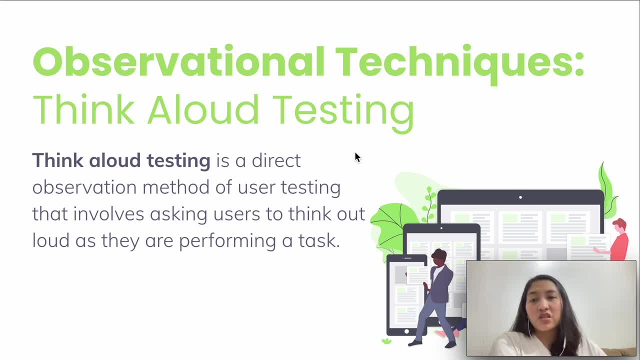 So this kind of evaluation technique has the advantage of simplicity, Because it requires little expertise to perform and can provide useful insight into the problems with an interface Okay. But there are also disadvantages in using this, because the process of observation can alter the way that people perform tasks and so provide a biased view. 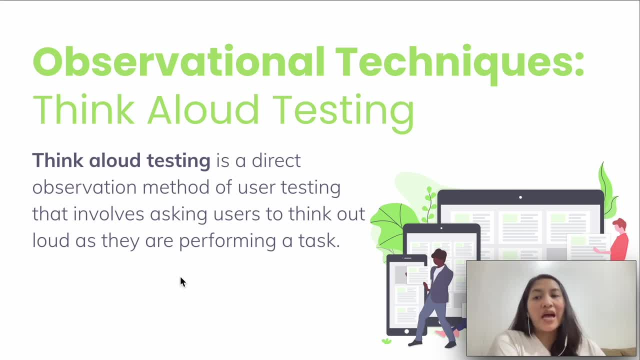 So it could be that the way they say things is not really what will happen in the actual usage of the system, Because the very act of describing what you are doing would not show the value from what you are doing or what you are moving along meaning if it is the only article. data you can see on the paper, or if it is the only text piece on the paper that you are going to see, Aha, so it doesn't matter that they are presenting or characterizing over the screen. This gives you the idea ofjan sh testament fui, the character system, but if you are monitoring oranges and 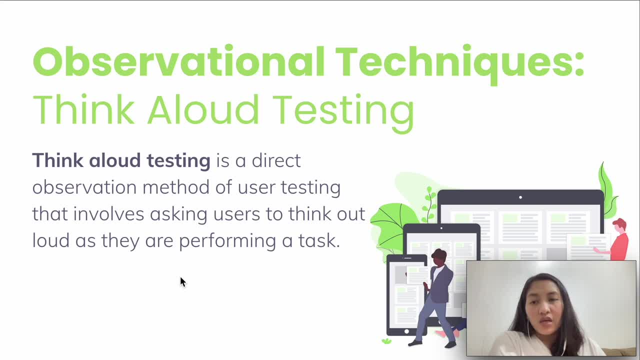 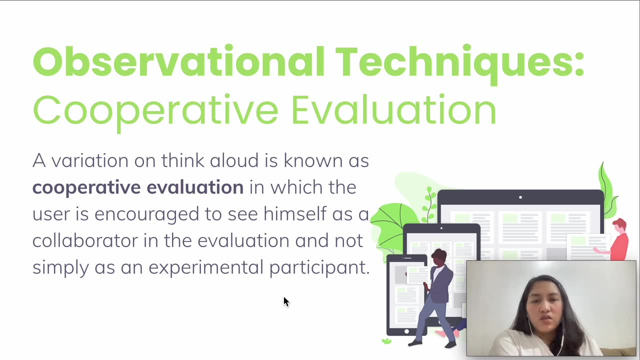 sh payment or CPA distribution or vậy-the-ה switching records and so on, of the same course of you are doing often changes the way you do it. so that's the disadvantage, this disadvantage over this technique. so that's why, in observational techniques, they have come up with what we call. 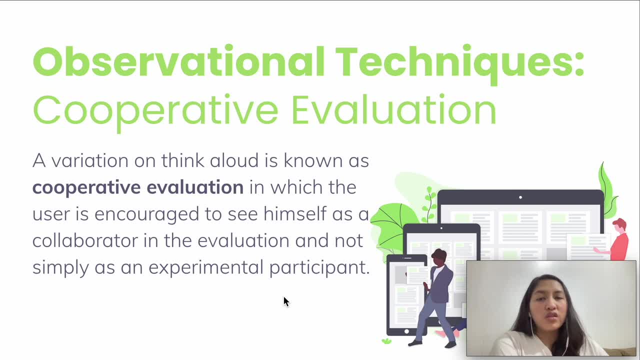 cooperative evaluation. this is a variation on think aloud in which the user is encouraged to see himself as a collaborator in the evaluation and not simply as an experimental participant. so here, as well as asking the user to think aloud at the beginning of the session, the evaluator can 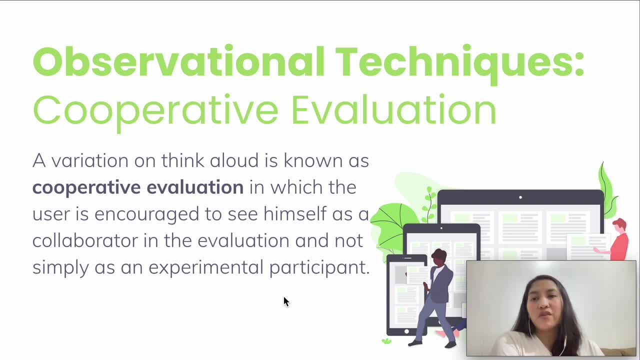 ask the user question. the user questions typically of the why or what, if type, if his behavior is unclear, and the user can ask the evaluator for clarification if a problem arises. so there are two actors here, um: the first one is the user and then the second one is the. 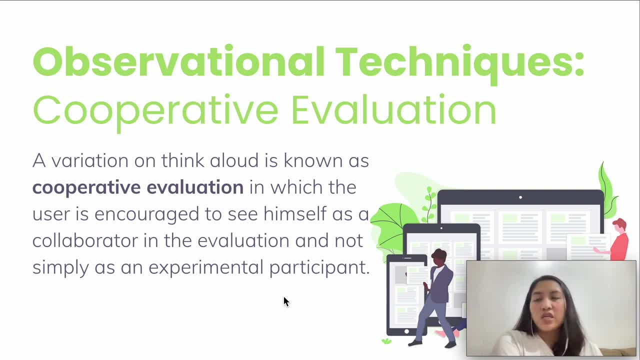 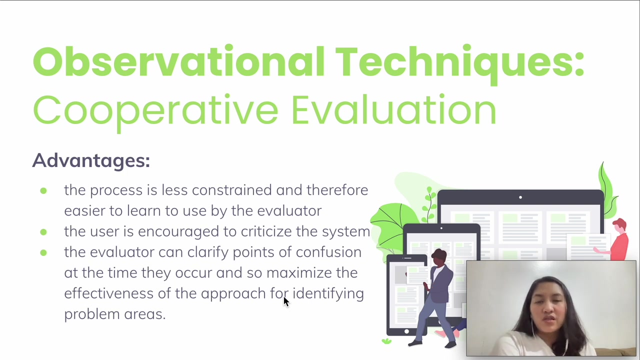 uh well, the expert on which he or she can ask questions from for clarification if the problem arises. so somehow the disadvantage to the think aloud will be eliminated, because it's as if the user is solving a problem and he is interacting with somebody else. so what are the advantages of this process? the cooperative evaluation. 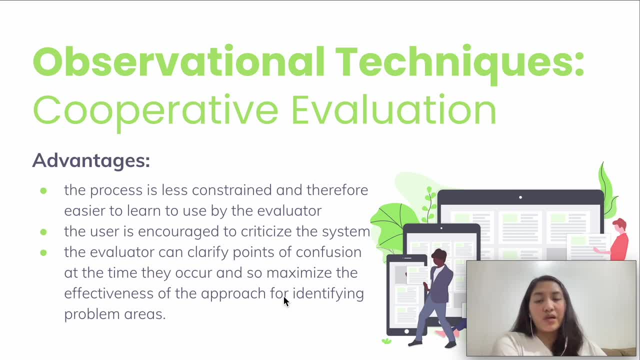 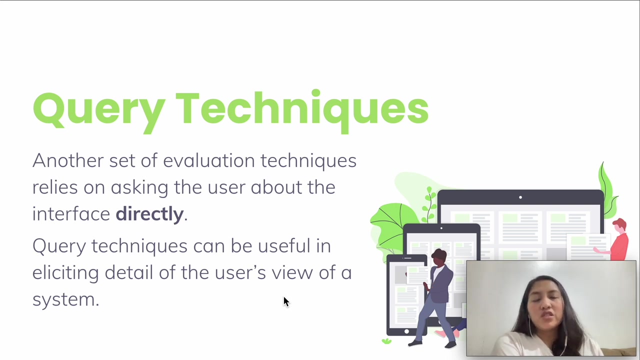 so the process is less constrained and therefore easier to learn to use by the evaluator. the user is encouraged to criticize the system. the evaluator can clarify points of confusion at the time they occur and so maximize the effectiveness of the approach for identifying problem areas. so now let's discuss about the query techniques, so another set of evaluation techniques by the 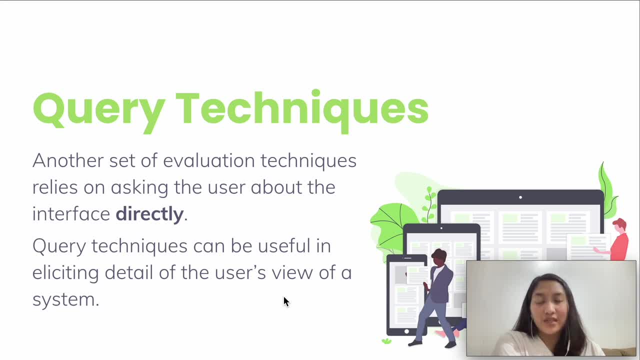 users rely on asking the user about the interface directly. query techniques can be useful in detail of the user's view of a system. so here the query techniques. it embody the philosophy that states that the best way to find out how a system meets user requirements is to ask the user they 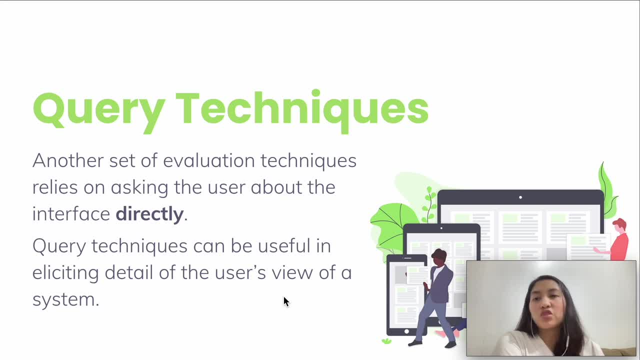 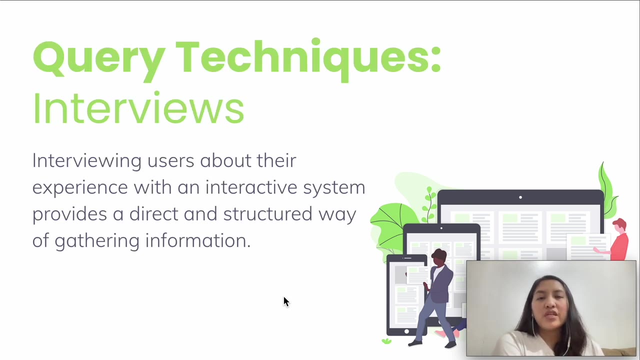 can be used in evaluation and, more widely, to collect information about user requirements and the task. the advantage of such methods is that they get the user's viewpoint directly and may reveal issues that have not been considered by the designer. so the first query technique is what we call interview. in interviewing users, 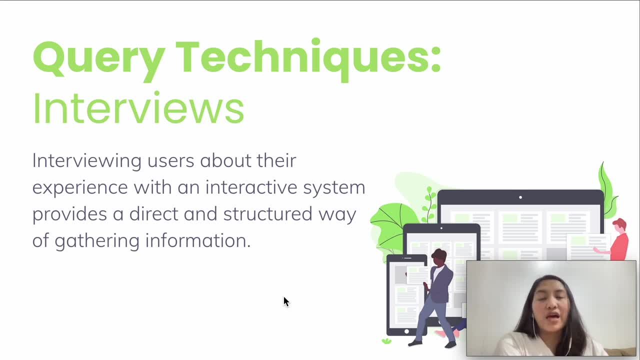 here the users are being interviewed about their experience with an interactive system. it provides a direct and structured way of gathering information. so interviews have the advantages that the level of questioning can be varied to suit the context and that evaluator can probe the user more deeply on interesting issues as they arise. 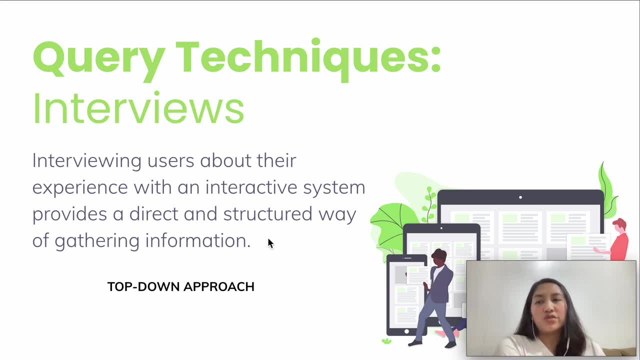 an interview will usually follow up a top-down approach, starting with a general question about a task and progressing to more leading questions, often in the form of why or what if, to elaborate aspects of the user's response. in order to be as effective as possible, the interview should be planned in advance with a set of central questions prepared. 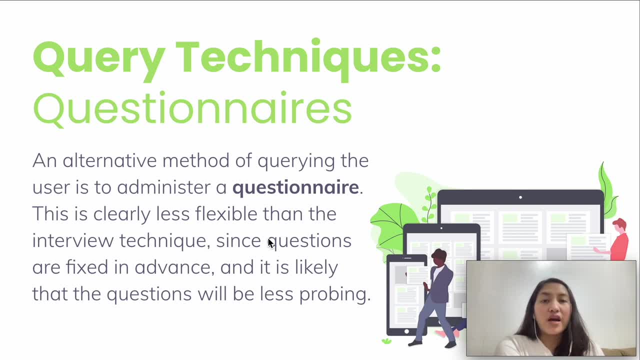 so an alternative method of querying the user is to administer a questionnaire. this is clearly less flexible than the interview technique, since questions are fixed in advance and it is likely that the questions will be less probing. so you cannot ask why unless you have provided it in the questionnaire itself. however, it can be used to reach a wider participant. 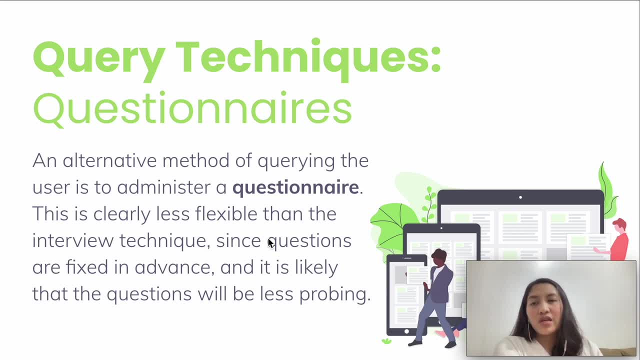 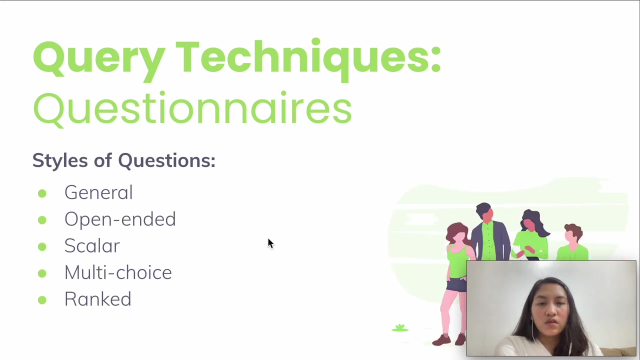 group. it takes less time to administer and it can be analyzed more rigorous. rigor, rigorously. it can also be administered at various points in the design process, including during requirements capture, task analysis and evaluation in order to get information on the user's needs, preferences and experience. so in questionnaires we have several types of questions or styles of questions. 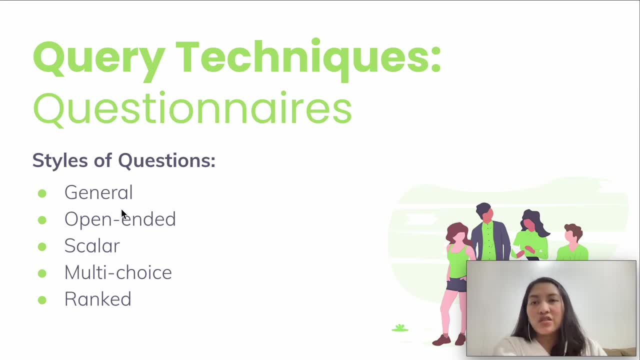 we have general, where these are the questions that help to establish the background of the user and his place within the user population. they include questions about age, gender, occupation, place of residence and so on. they may also include questions on previous experience with computers, which may be praised as open-ended, multiple choice or scalar questions. 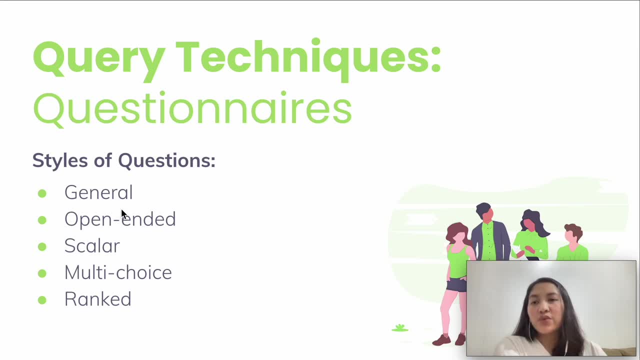 so when you say open-ended, this asks the user to provide his own unprompted opinion on a question, for example. can you suggest any improvements to the interface? they are useful for gathering general subjective information, but are difficult to analyze in any rigorous way or to compare, and can only be viewed as supplementary. so the third style of question. 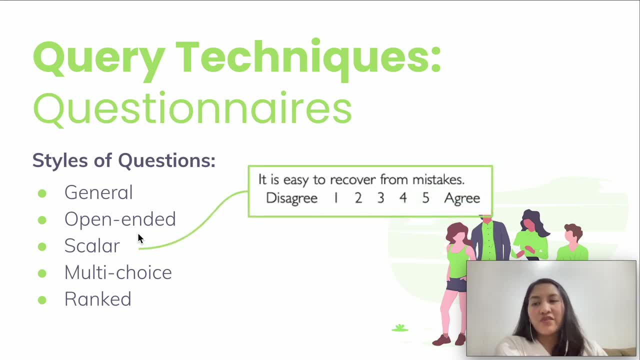 is what we call scalar. this asks the user to judge a specific statement on a numeric scale as what we can see in the example, usually corresponding to a measure of agreement or disagreement with a statement. so we also have multiple choice or multi-choice, where the respondent is offered a choice of explicit responses. 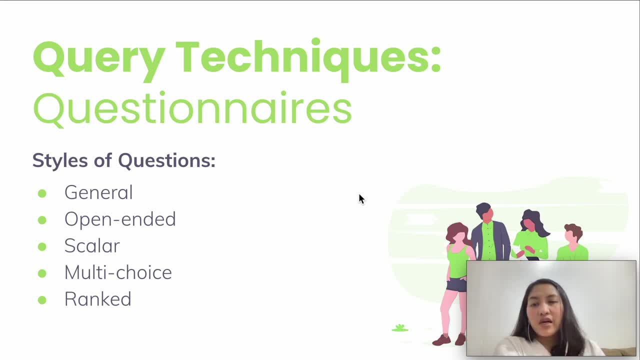 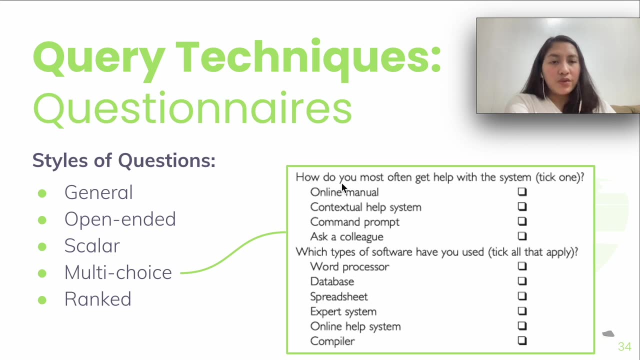 and we have a lot of different options to select only one of this or as many as apply. so here is an example. okay, so we have here a question about how do you most often get help with the system or which type of software have you used. so this is an example of a multiple or multi-choice. 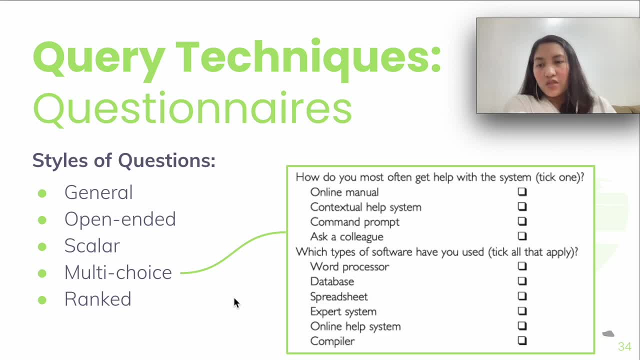 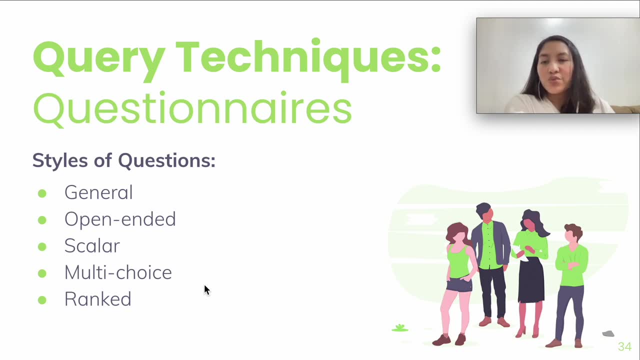 style of questions- and lastly, we have rant, so this plays an ordering on- and are useful to indicate a user's preferences. So we have here an example, A question such as: please wrap the usefulness of these methods of issuing a command. So there, those are the different styles of questions that you can use for, if you will. 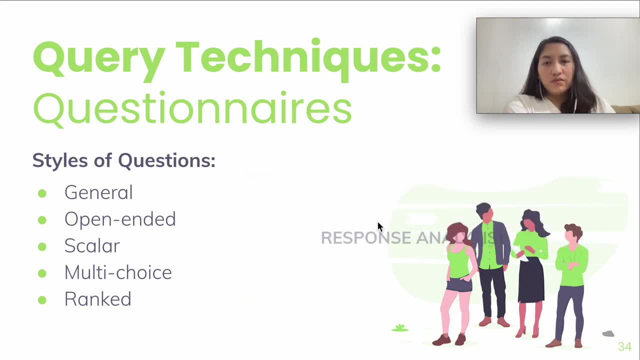 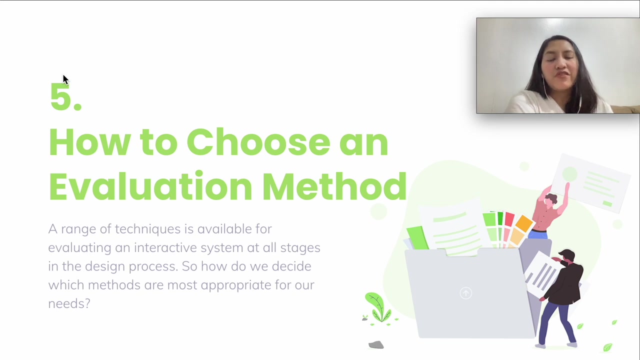 be administering questionnaires. Okay, so the responses can be analyzed in a number of ways, from determining simple percentages for each response to looking at correlations and factor analysis. So there are different methods available to analyze the response of users, mostly mathematical. So how to choose an evaluation method? a range of techniques is available for evaluating. 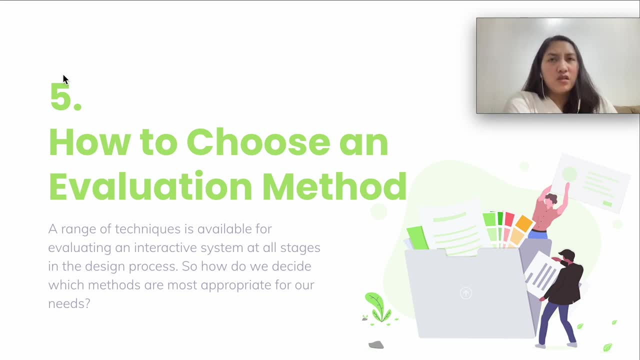 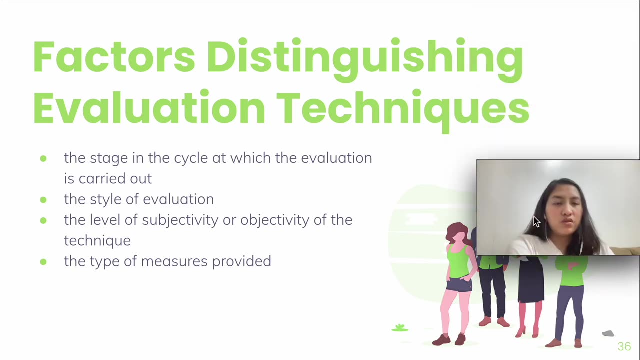 an interactive system at all stages in the design process. So how do we decide which methods are most appropriate for our needs? We have several factors to consider, So the first one is the stage in the cycle at which the evaluation is being carried out. 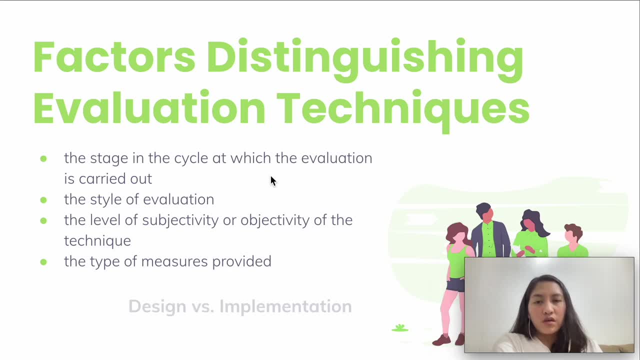 So you have to choose between design versus implementation, during the design or during the implementation. So, with that in mind, whether you are at which stage in the cycle, you have to consider which evaluation technique is the most appropriate. Second is the style of the evaluation. 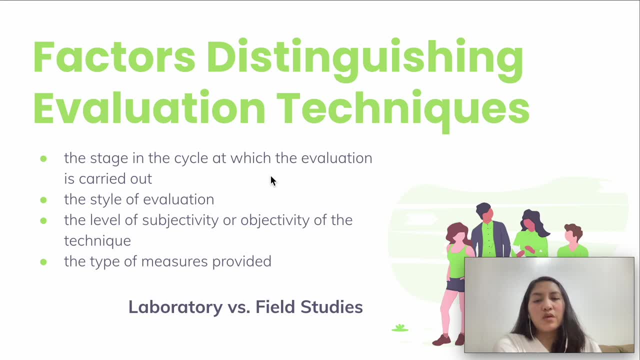 So will you use a laboratory setup or will you go there to your users to conduct field studies? So there are different pros and cons for each style of evaluation. In a laboratory setting there's a controlled experimentation and observation. So here you're using the naturalness of the user's environment, while in the field studies 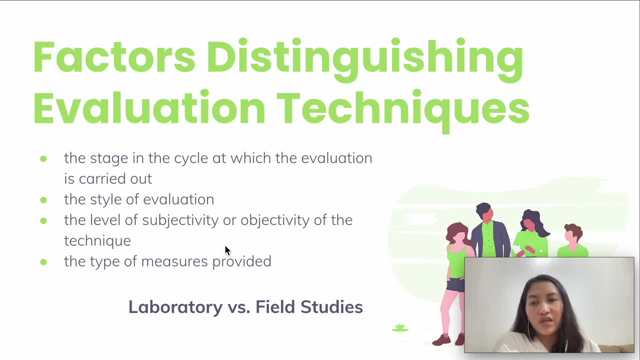 you can retain the naturalness of the user's environment, but you don't have any control over their activities. However, both styles of evaluation both has advantages and disadvantages. Third, the level of subjectivity or objectivity. So, as I said, the level of subjectivity is the highest. 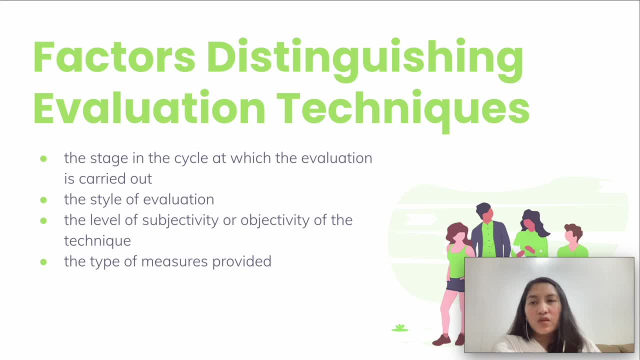 of the technique. So there are pros and cons among these two. So you have to choose between the result being subjective or the result being objective. So in an interview, probably the data that you can gather are more subjective than objective, while in the questionnaires it's more. 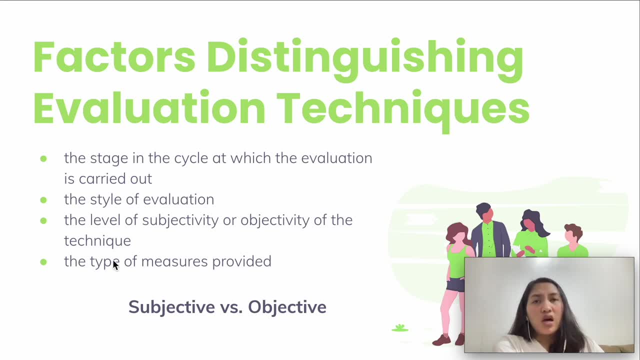 objective than subjective. So it depends on the level of expertise in the analysis of the results. So the third or the fourth is the type of measures provided. So in every evaluation technique you can gather different data. So we have quantitative versus qualitative measures. 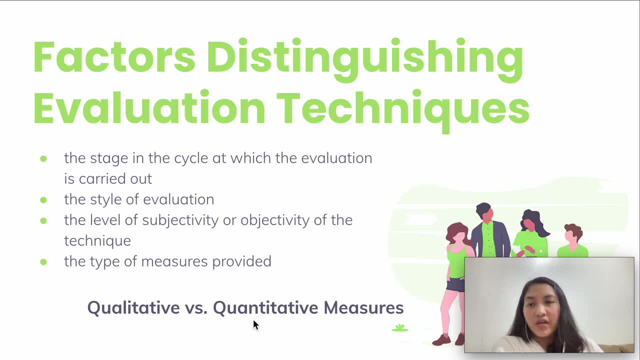 So the quantitative is the numeric And then the other one is non-numeric. So you have to choose which. do you need? the qualitative type of data or the quantitative type and analysis of the data? Next, the information provided. This is the level of information required from an evaluation. 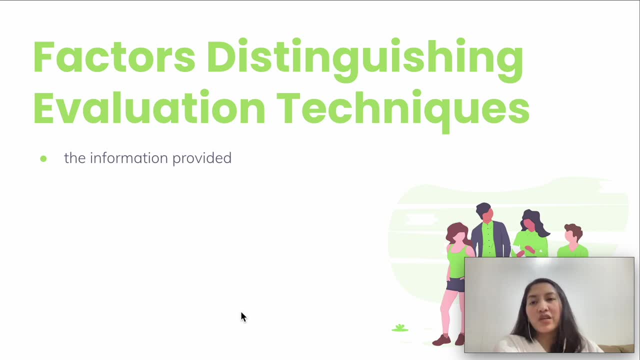 It can vary, Like the information required by an evaluator at any stage of the design process may range from low-level information to high-level information. The low-level information example is the font-that is most readable. That's the example, And the higher-level information is: is the system-usable? 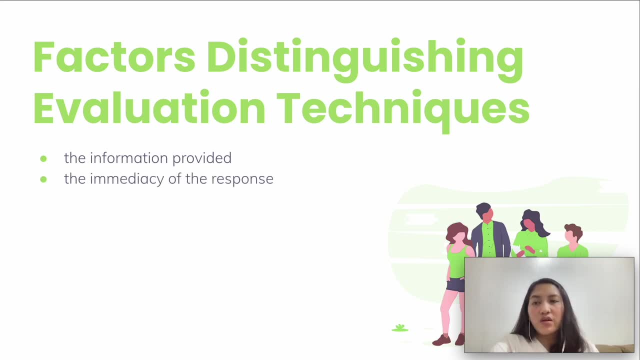 And then we also have the emergency of the response. So here this is another factor distinguishing evaluation technique. Some methods, such as think-aloud, record the user's behavior at the time of the interaction itself. Others, such as the post-task walkthrough, rely on the user's recollection of events. 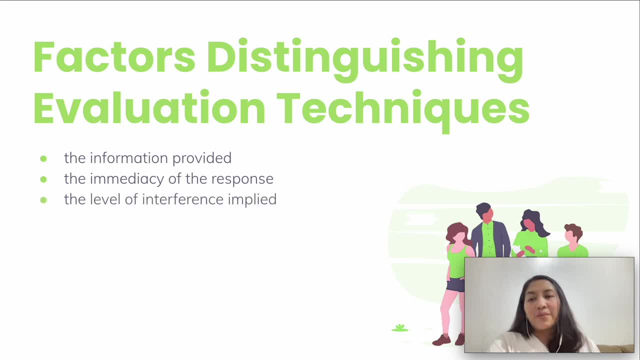 And then we also have the level of interference implied. So related to the immediacy of the response is the intrusiveness of the technique itself. Yung ibang techniques, particularly those that produce immediate measurements, are obvious to the user during the interaction. 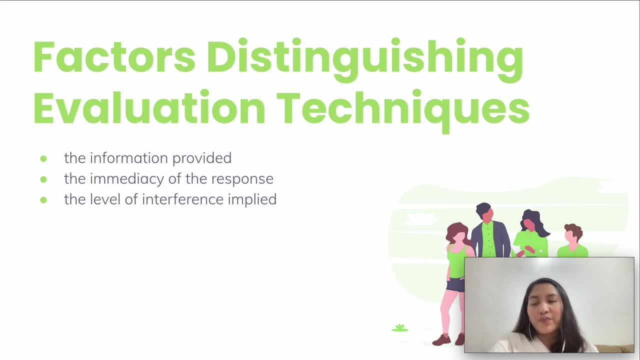 And therefore run the risk of influencing the way the user behaves. Sensitive activity on the part of the evaluator can help to reduce this, but cannot remove altogether. Most immediate evaluation techniques are intrusive, with the exception of automatic system logging. Unfortunately, this is limited in the information that it can provide and is difficult to interpret. 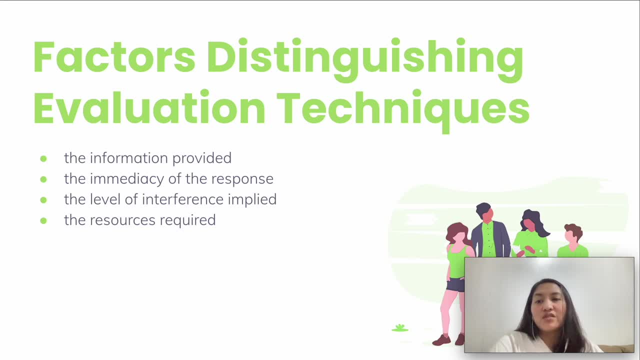 And, lastly, the resources required. This is the final consideration when selecting an evaluation technique. The resources to consider include equipment, time, money, participants, expertise of the evaluator and context. In some cases, the decisions are forced by resource limitations. 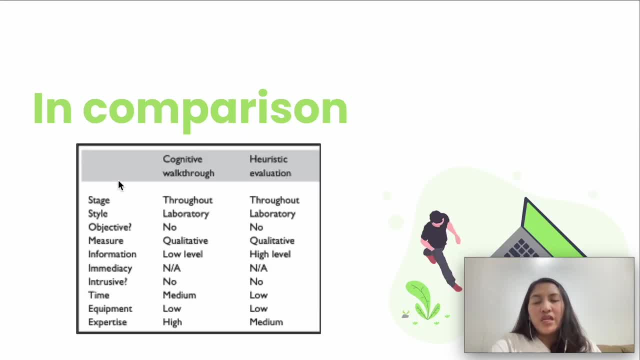 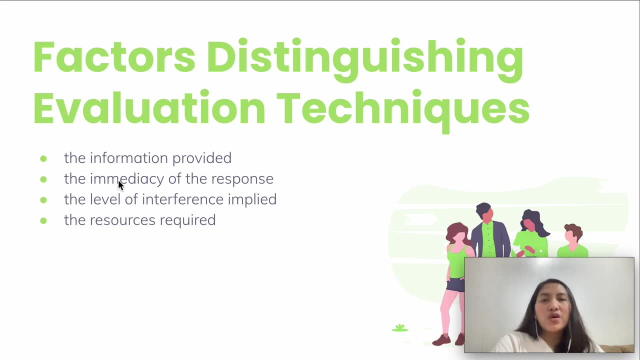 However, you really have to think which is the more important. Will you pay higher price for a better result or it's not important at all, because you can elicit information from other evaluation techniques that are available. that doesn't necessarily require a lot of effort. 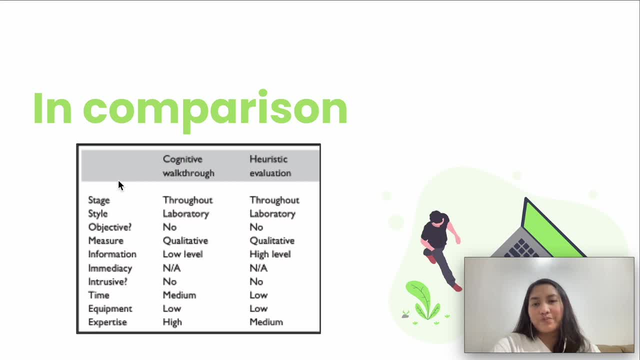 Because it is not necessarily to buy more expensive resources In comparison. you can use cognitive walkthrough and heuristic evaluation all through all the stages, both or in a laboratory setting, Both are subjective, Both measures or both evaluation techniques produces or produce qualitative results to improve the evaluation of the potential result to be obtained. 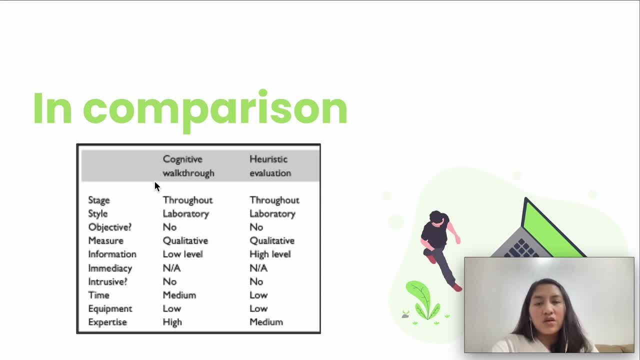 produces or produce qualitative results to improve the evaluation of the potential results to be obtained. data and the information that you can get in a cognitive walkthrough is low level, while in heuristic evaluation it's higher level. The emergency is not applicable intrusiveness: both are no, and then the time needed for. 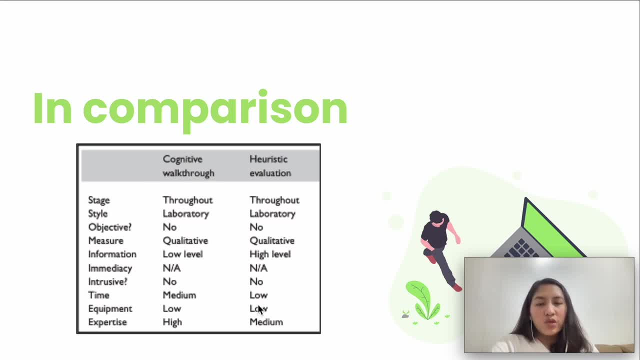 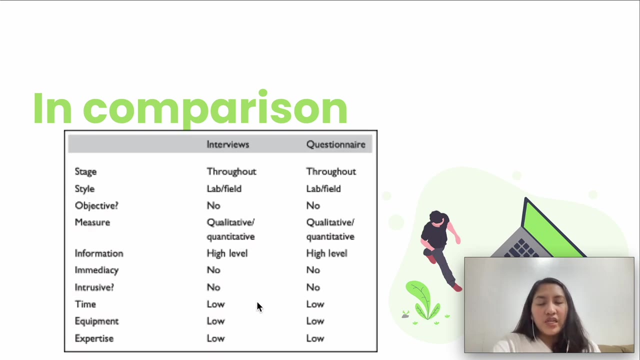 the cognitive walkthrough is medium, while the heuristic evaluation is low. The equipment: both are low. it doesn't require much, while the expertise for cognitive walkthrough is high, while in heuristic evaluations it's in the middle. For the interviews and questionnaire you can also use this all throughout the design. 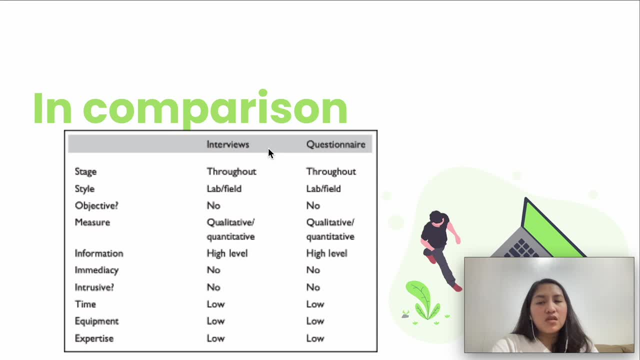 stage or the development stage, while the style for interviews and questionnaires can be both in lab or in the field- Both of them- you can have subjective answers. While the measure for both techniques can be qualitative, you can get qualitative and quantitative data. 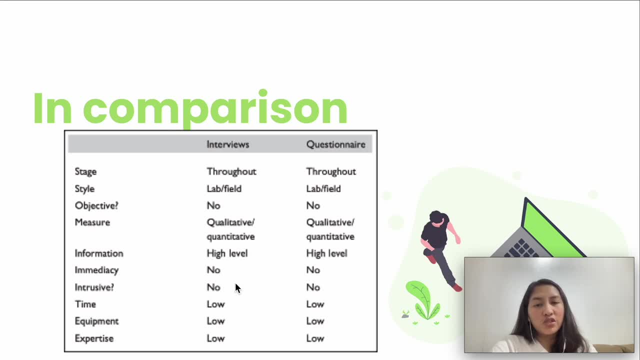 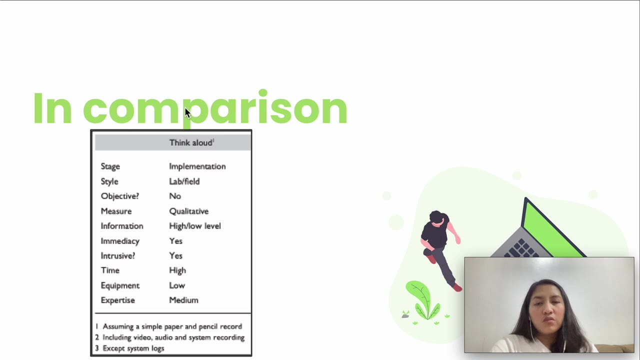 For the information. both of them elicit high-level information and for the time, it requires low equipment and expertise. also, You can also check on the module about the think aloud. We can apply this during the implementation. It can be done either in the lab or in the field.